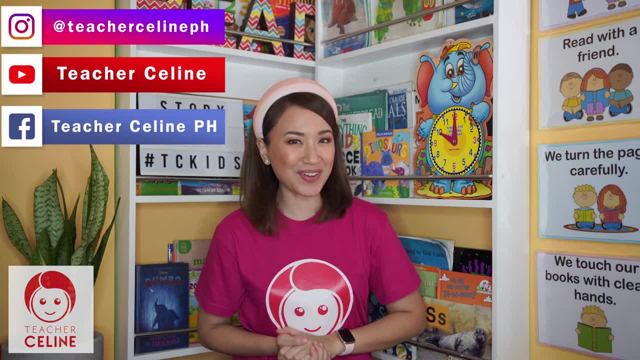 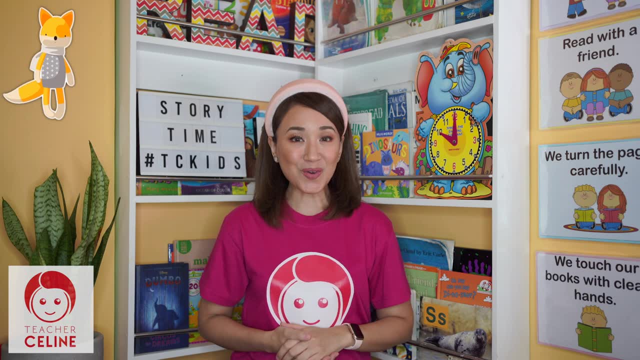 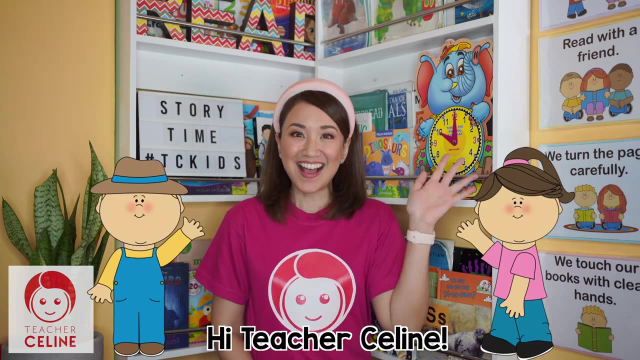 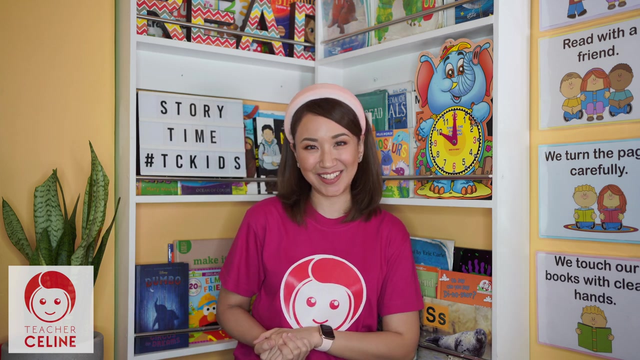 Hi TC Kids. How are y'all doing? Oh, you know what? Teacher Celine is so happy to see you again. Oh, if you're new to my channel, my name is Teacher Celine. Can everybody say: Hi, Teacher Celine, And welcome to my online learning channel. 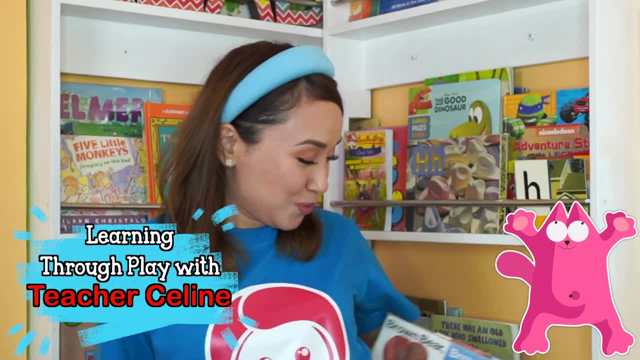 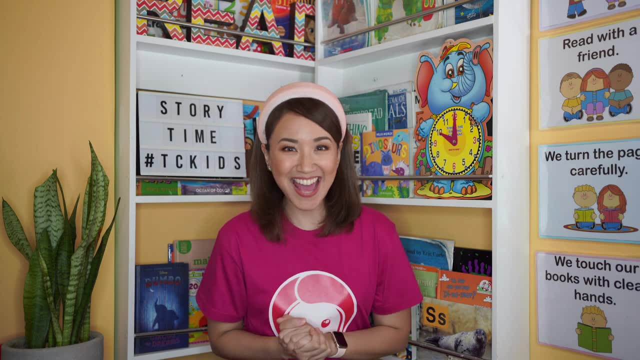 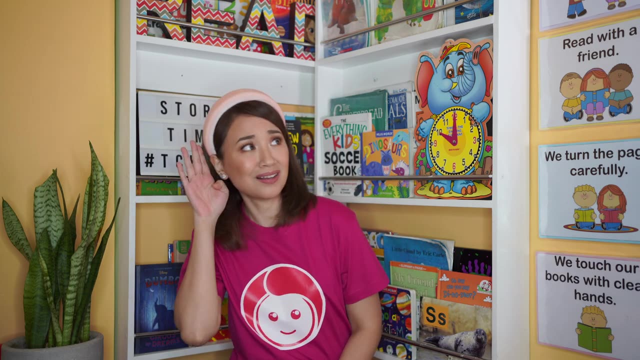 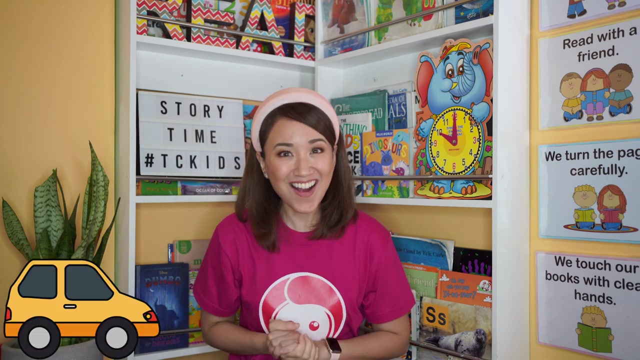 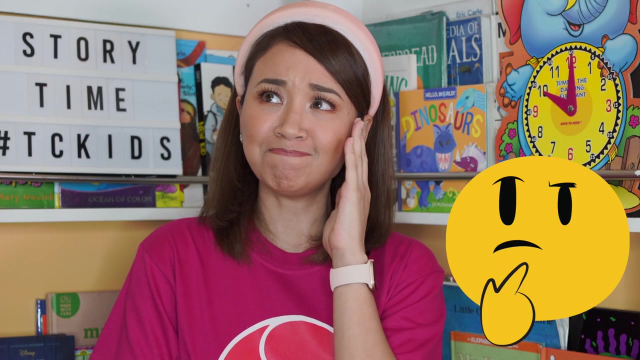 You know what kids Today wait a minute. Do you hear that sound? What sound is that? I think it's a car. Do you think it's a car? No, Hmm, Aha, I think those are footsteps. 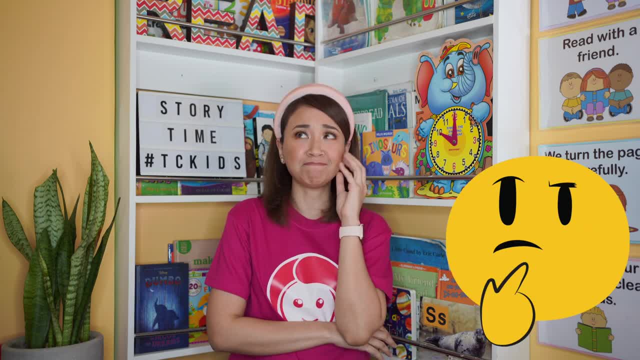 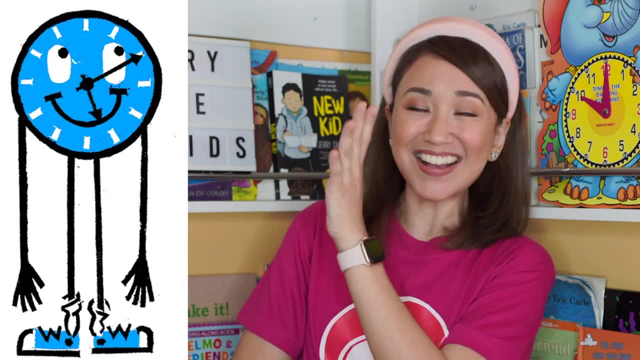 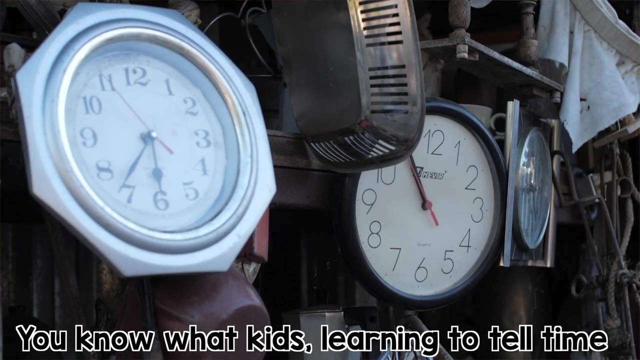 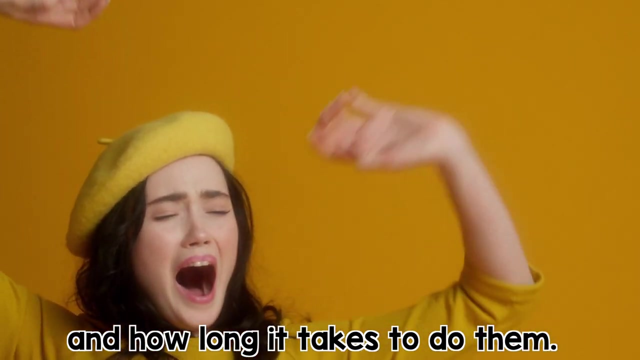 Nope, Hmm, Oh look, Say Hi, Mr Clock. Today's lesson is about telling time. You know what kids Learning to tell time is a very important skill to have, so you know when to do specific activities and how long it takes to do them. 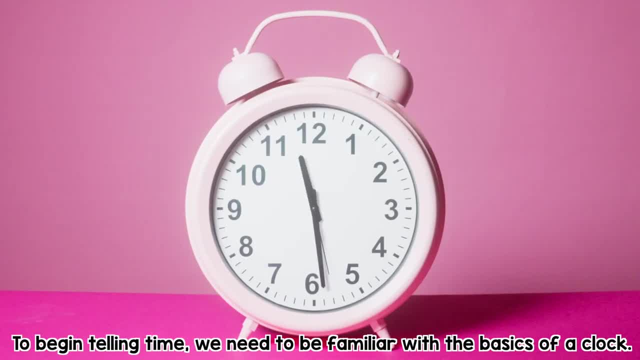 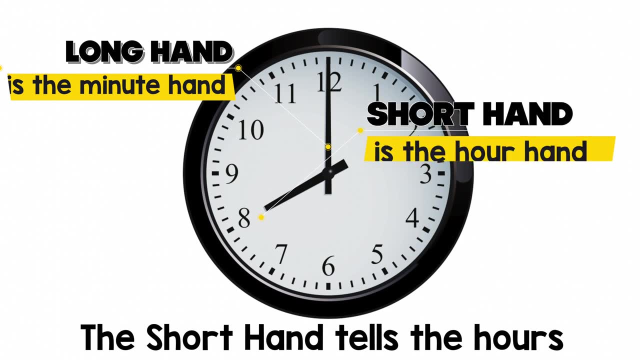 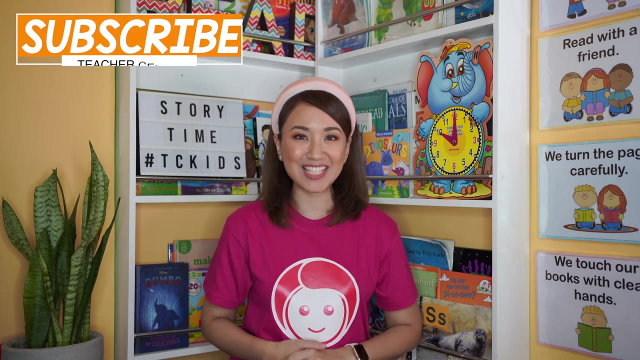 To begin telling time, we need to be familiar with the basics of a clock. The long hand tells the minutes. The short hand tells the hours. Before our story time, let's sing a song. This song is a good one for you to learn about telling time. 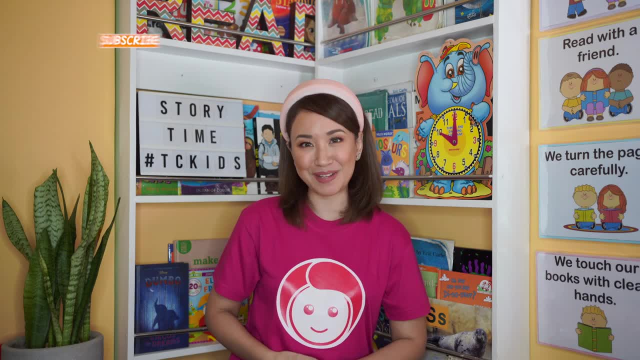 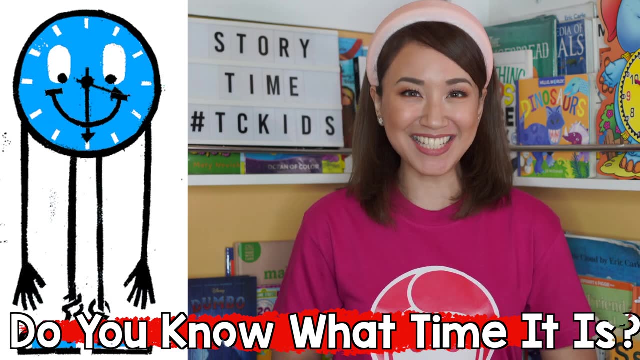 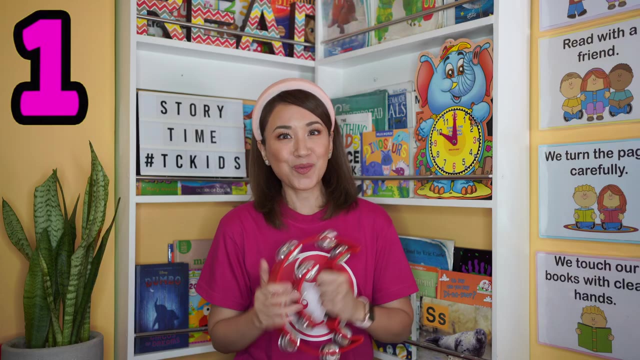 If you have any instruments, please get them now. Now the title of the song is: Do You Know What Time It Is? Don't worry, TC kids, This will be really easy. Just follow Teacher Celine Ready. One, two, three go. 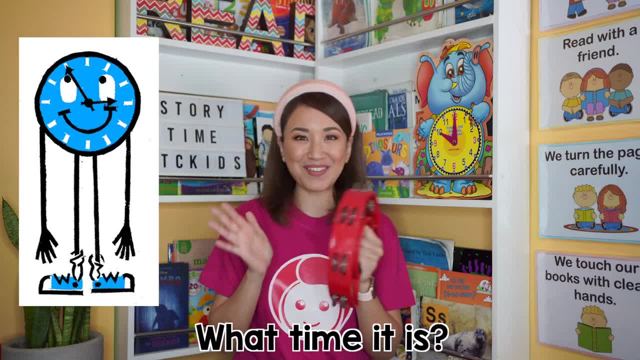 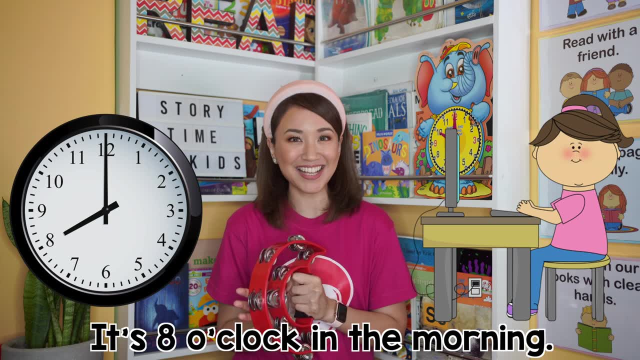 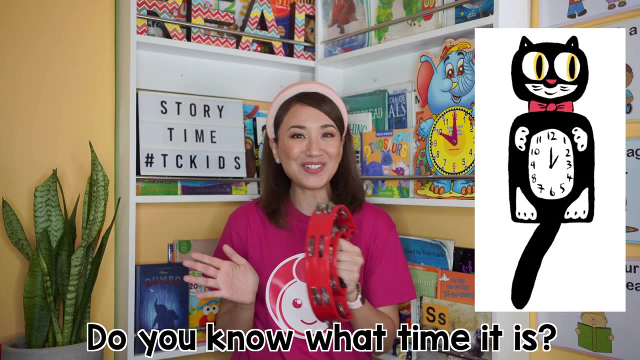 Do you know what time it is, What time it is, What time it is? Do you know what time it is? It's eight o'clock in the morning. Do you know what time it is? It's four o'clock in the afternoon. 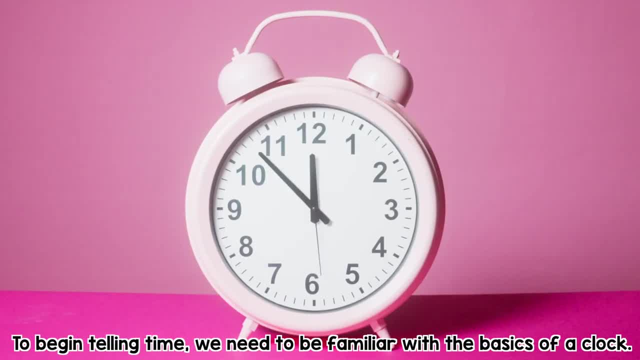 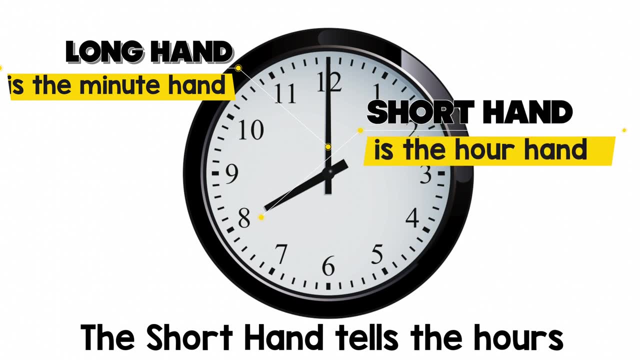 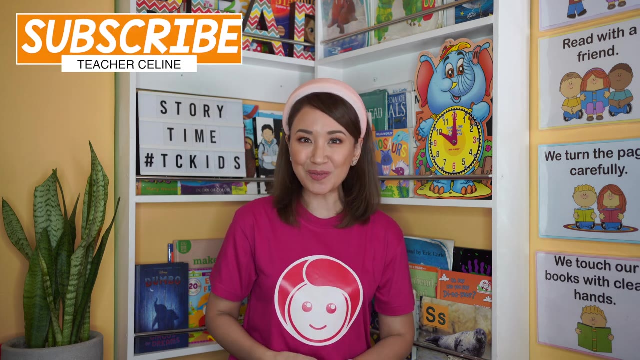 To begin telling time, we need to be familiar with the basics of a clock. The long hand tells the minutes. The short hand tells the hours. Before our story time, let's sing a song. This song is a good one for you to learn about telling time. 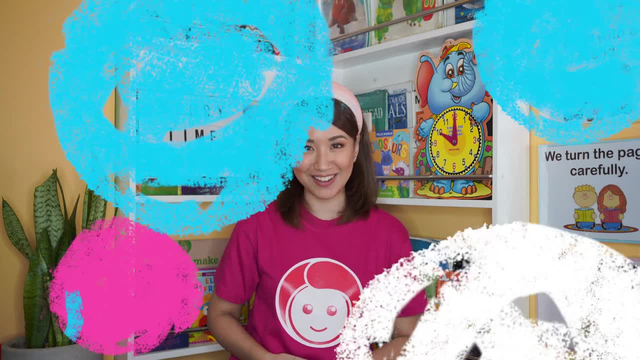 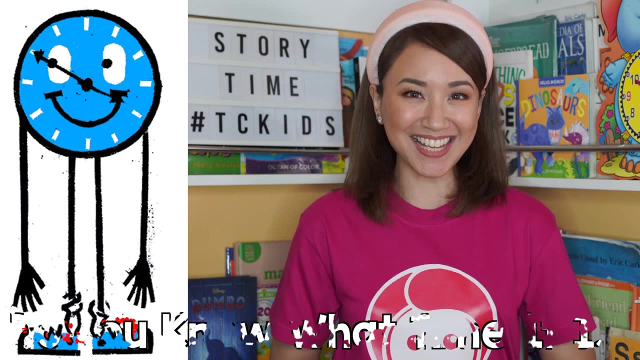 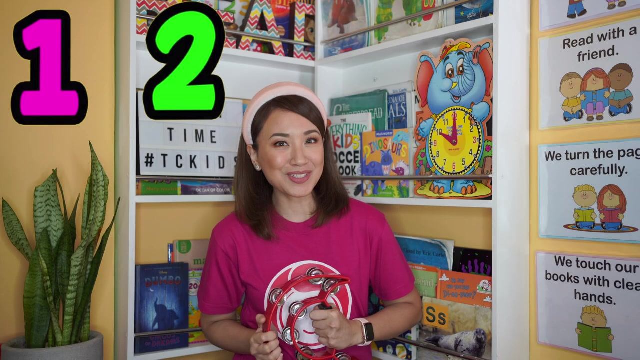 If you have any instruments, please get them now. Now the title of the song is: Do You Know What Time It Is? Don't worry, TC kids, This will be really easy. Just follow Teacher Celine Ready. One, two, three go. 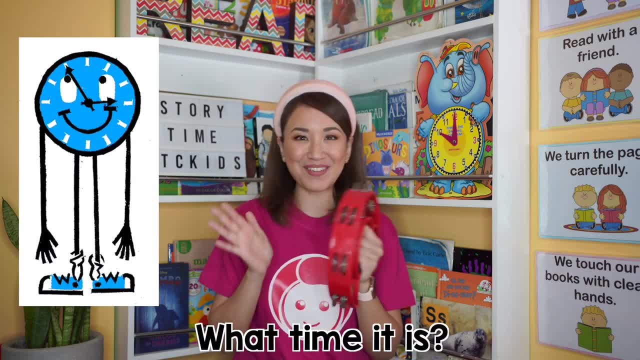 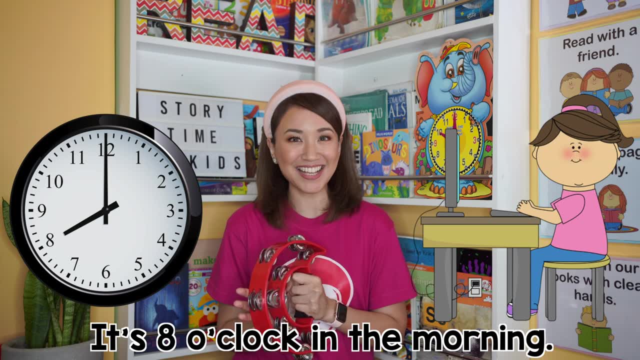 Do you know what time it is, What time it is, What time it is? Do you know what time it is? It's eight o'clock in the morning. Do you know what time it is, What time it is, What time it is? 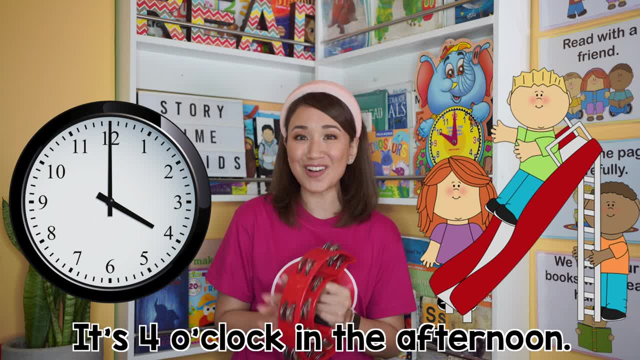 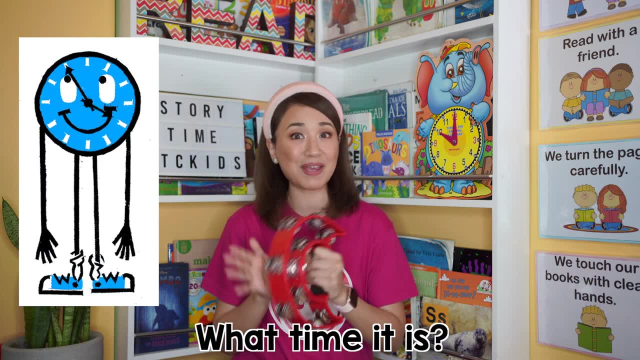 Do you know what time it is? It's four o'clock in the afternoon. Do you know what time it is, What time it is, What time it is? Do you know what time it is? It's seven o'clock in the evening. 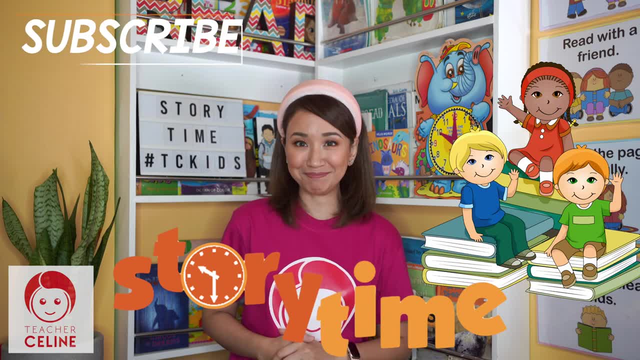 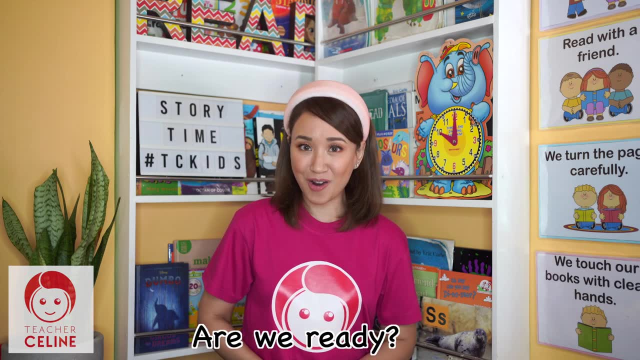 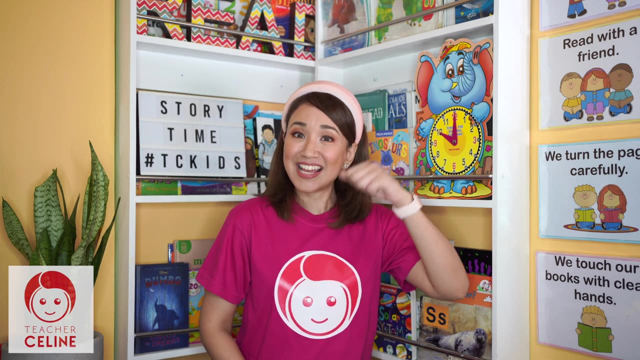 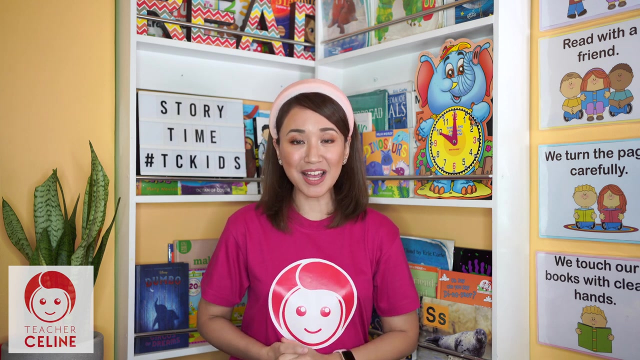 Are you ready for story time? Hmm, let me check if you are ready. When Teacher Celine says: Are we ready, Are we ready? You will answer: Yes, we are, Yes, we are. Can we do that one more time? 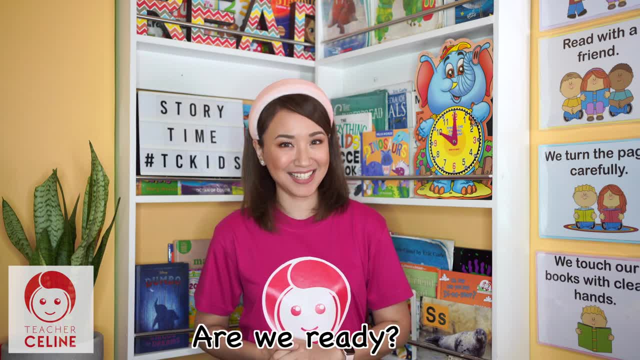 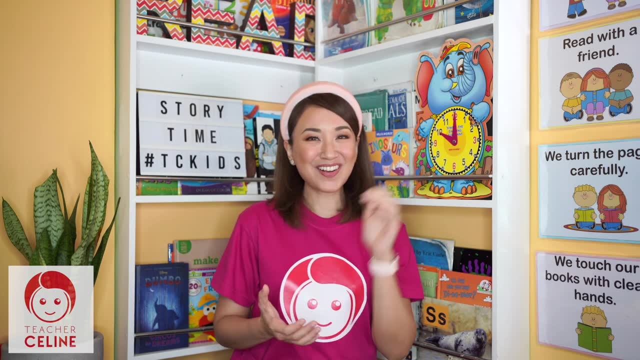 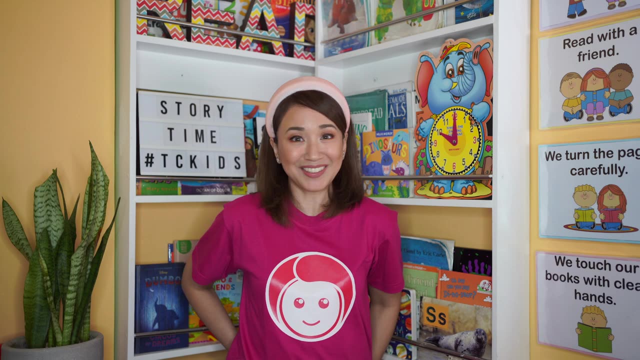 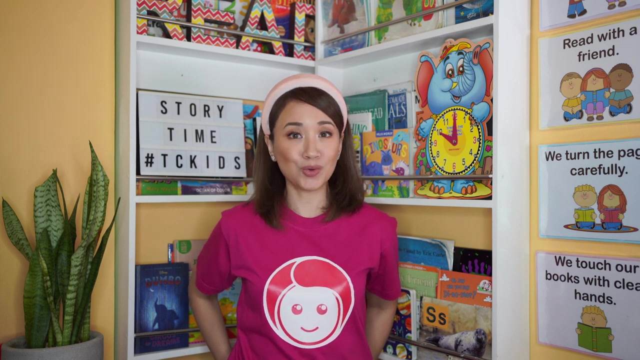 One, two, three go. Are we ready? Are we ready? Yes, we are. Yes, we are. Great job. Let me get my book. I have a story. what could it be? Whoop, I have a story. who could it be? 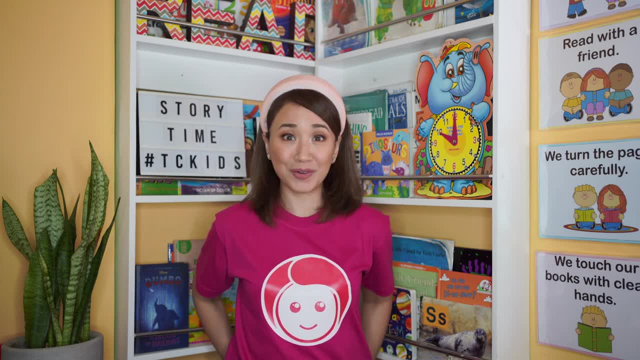 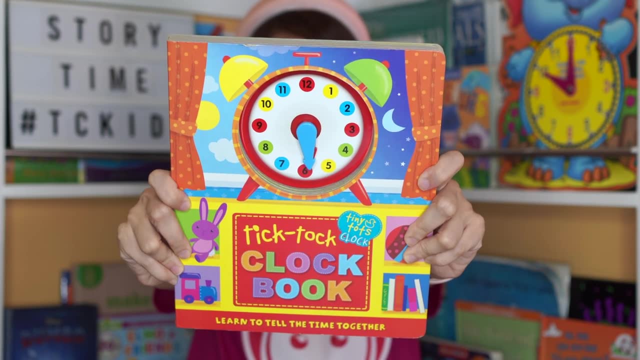 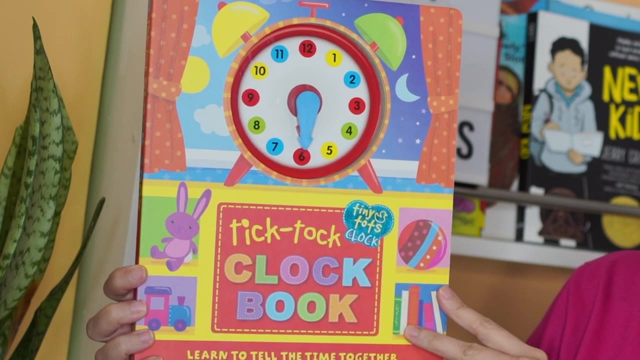 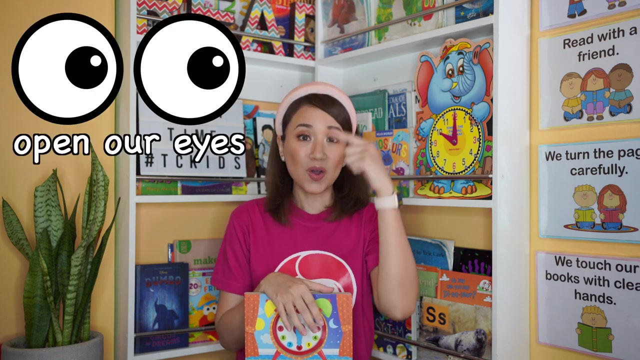 Whoop. I have a story. what could it be? Whoop? The title of the story is Tick Tock Clockbook. When Teacher Celine is reading a story, what should we do? We should open our eyes, Open your eyes. 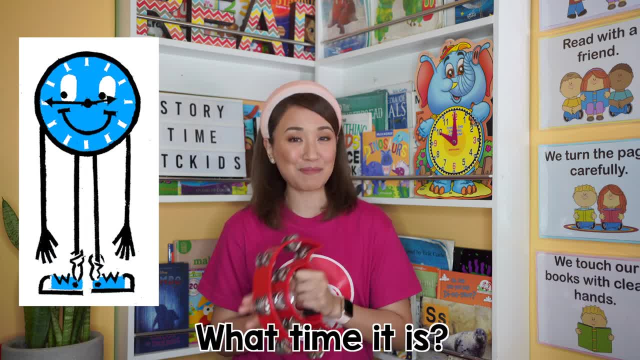 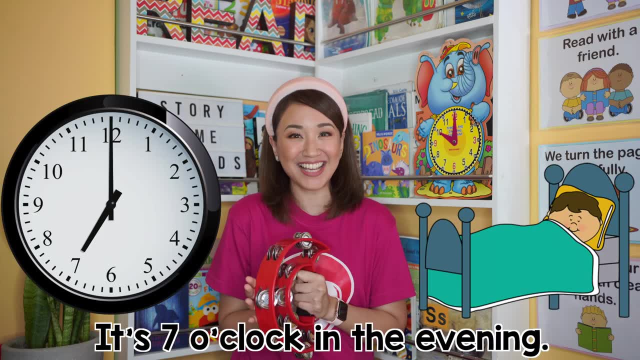 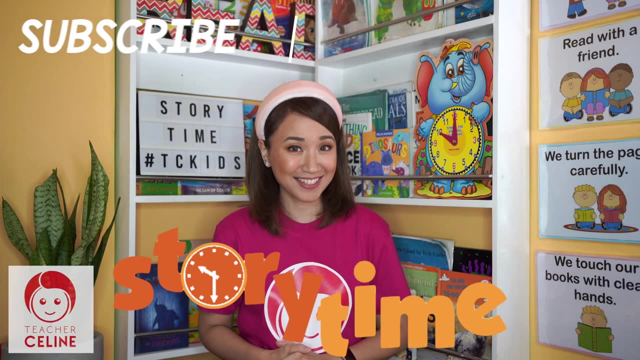 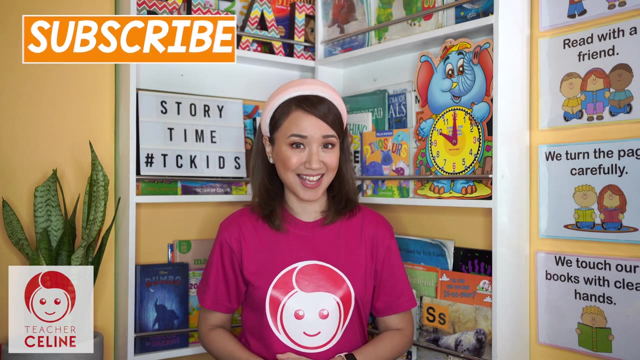 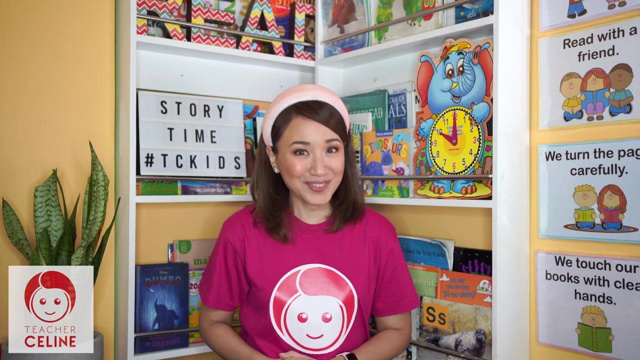 Do you know what time it is? It's seven o'clock in the evening. Are you ready for story time? Yay, Hmm, let me check if you are ready. When Teacher Celine says, are we ready, Are we ready, You will answer yes, we are. Yes, we are. 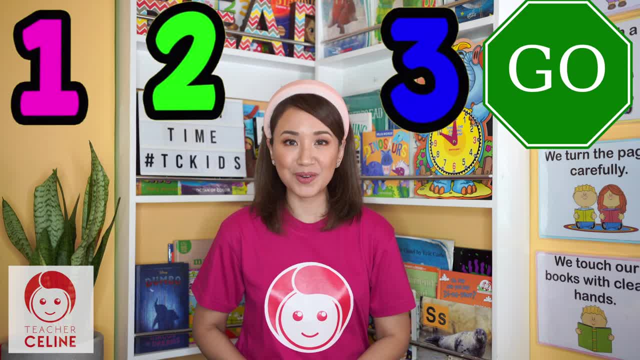 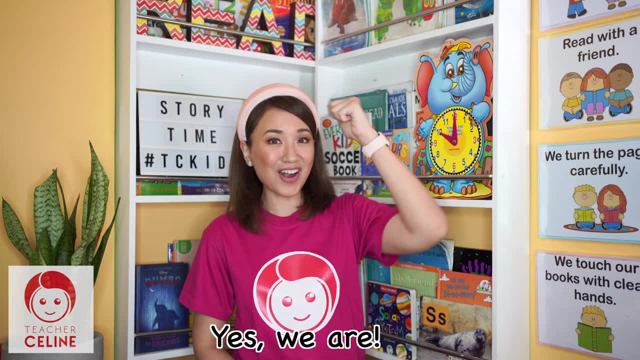 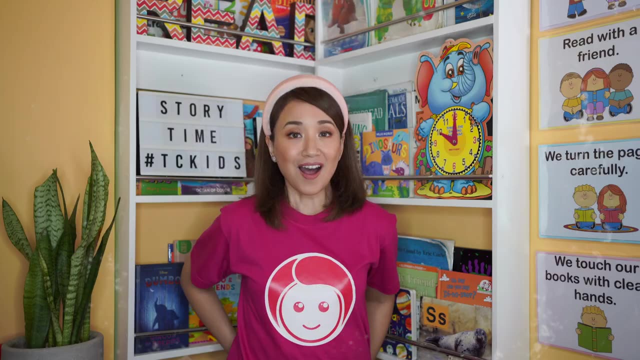 Can we do that one more time? One, two, three go. Are we ready? Are we ready? Yes, we are. Yes, we are. Great job. Let me get my book. I have a story. what could it be? 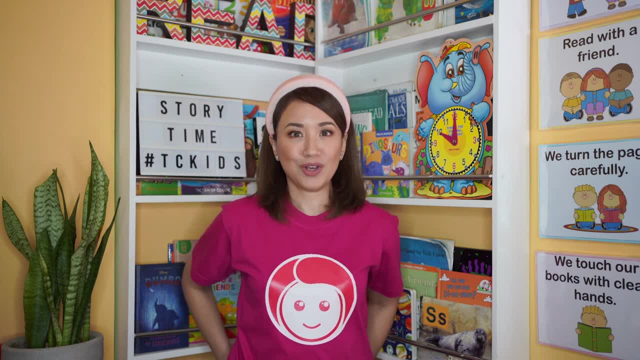 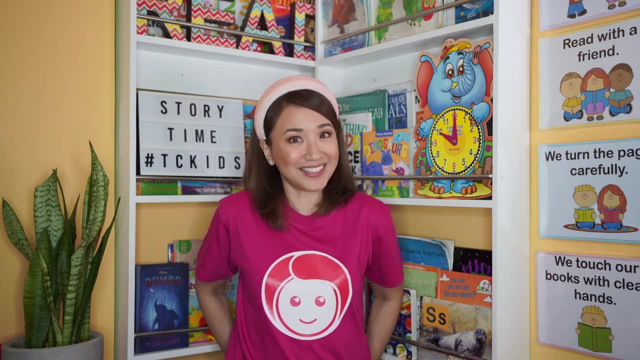 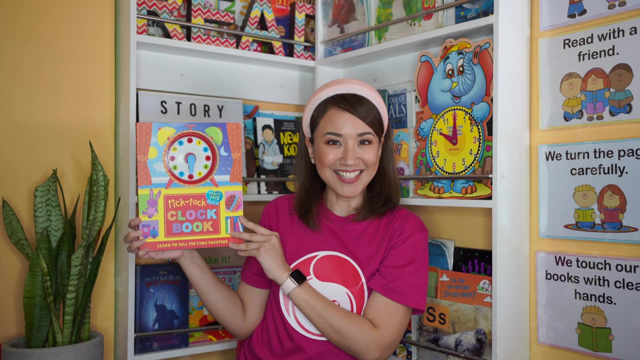 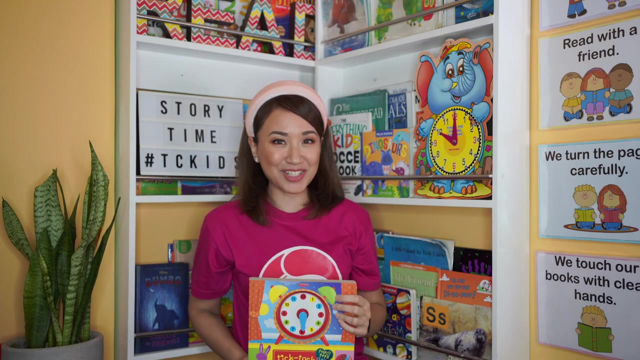 I have a story. who could it be? I have a story. what could it be? What could it be? Ta-da, The title of the story is Tick-Tock Clockbook. When Teacher Celine is reading a story, what should we do? 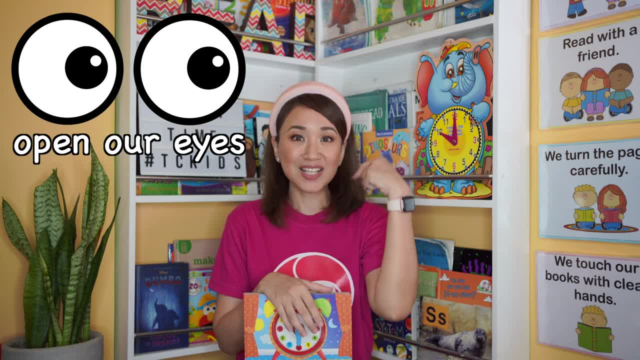 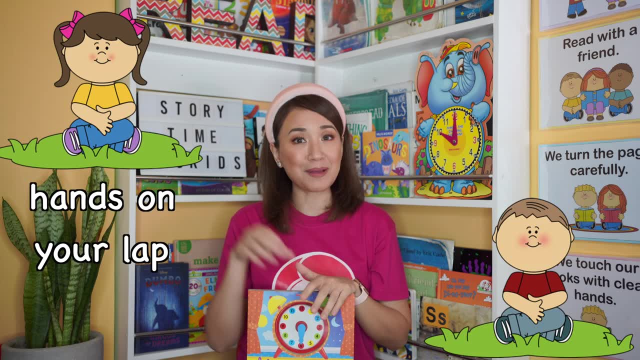 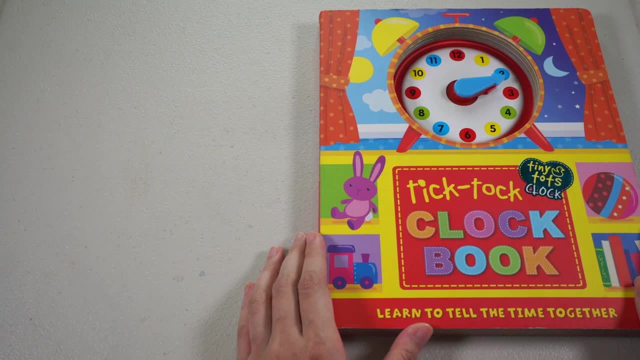 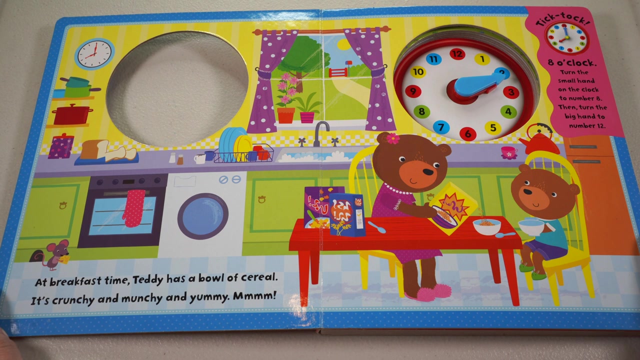 We should open our eyes, open your eyes, open our ears, lock our lips. hands on our lap, Sit like a pretzel and eye on the book- Tick-Tock Clockbook. At breakfast time, Teddy has a bowl of cereal. 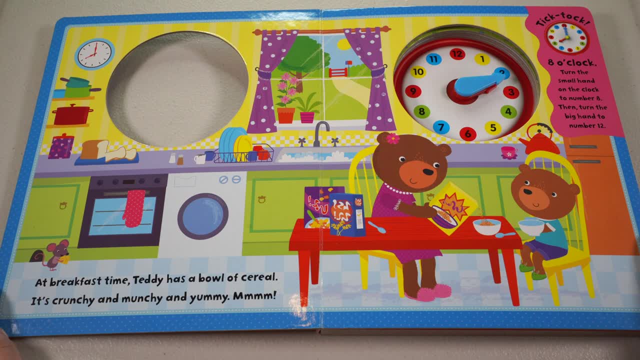 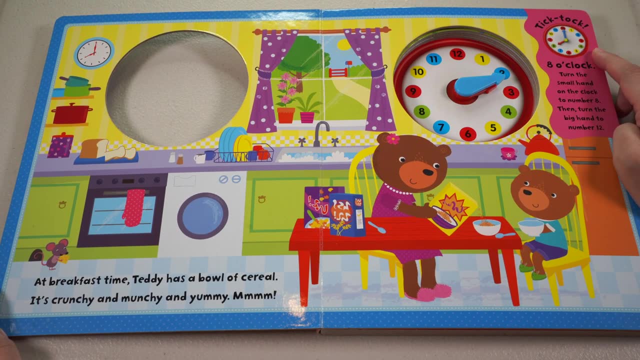 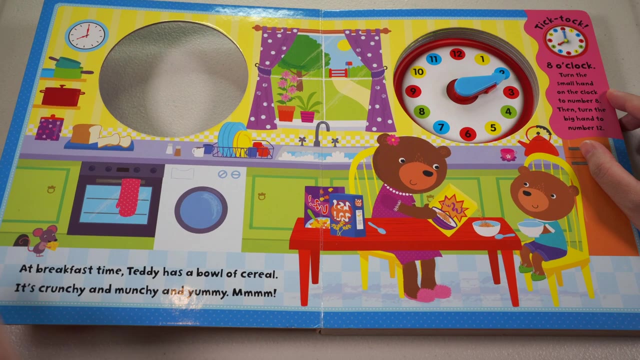 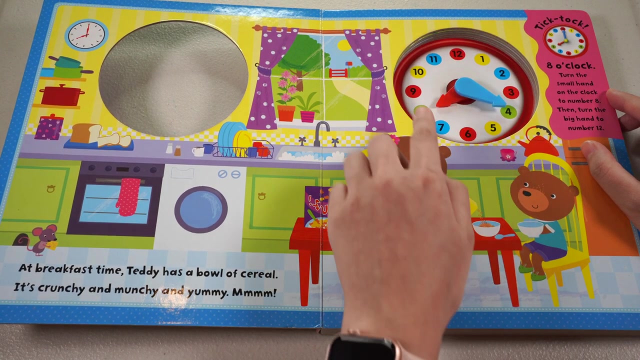 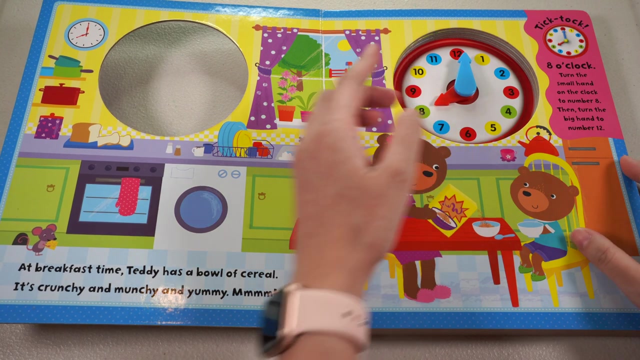 It's crunchy and munchy and yummy. Tick-tock, tick-tock, it's eight o'clock. Turn the small hand on the clock to number eight. Then turn the big hand to number twelve. Ta-da, It's eight o'clock. 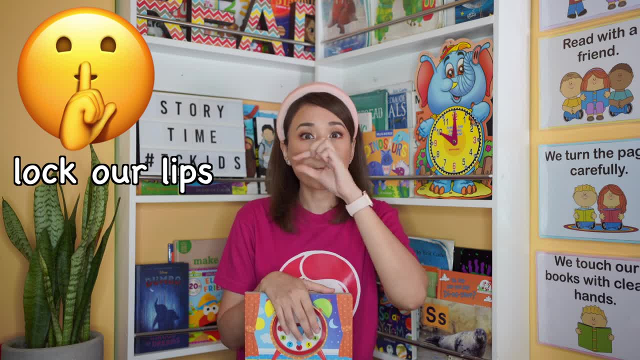 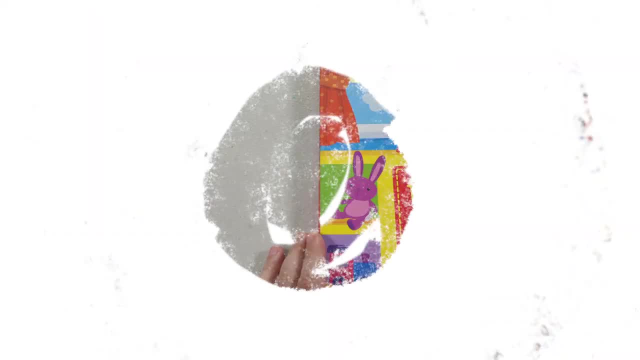 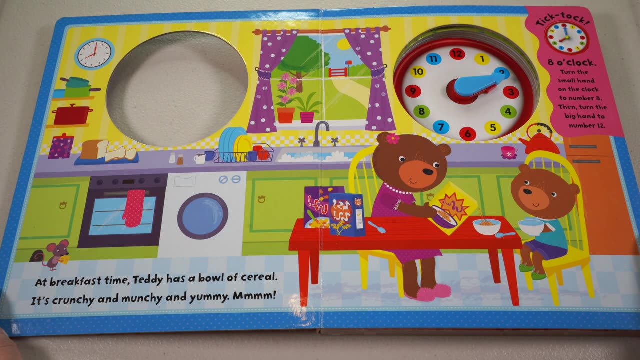 Open our ears, Lock our lips. Hands on our lap Sit like a pretzel and eye on the book, Tick, tock Clockbook. At breakfast time Teddy has a bowl of cereal. It's crunchy and munchy and yummy. 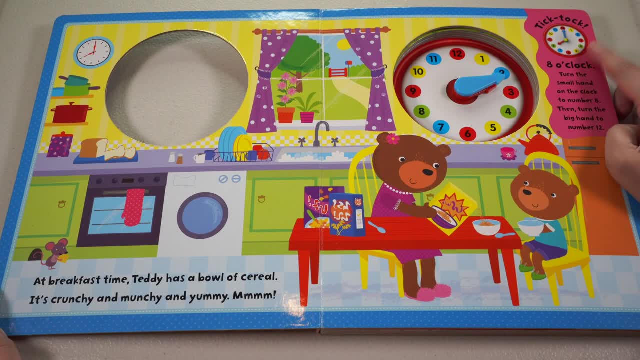 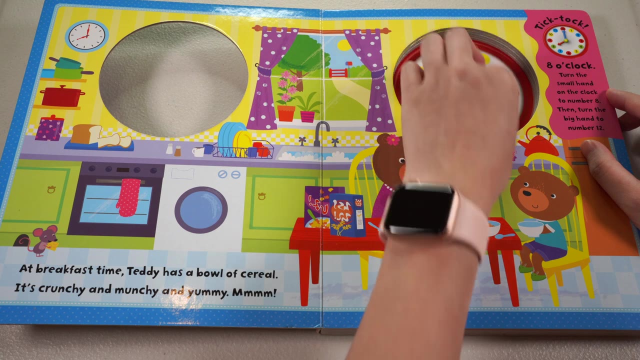 Mmm, Tick tock, Tick tock. It's eight o'clock. Turn the small hand on the clock to number eight. Tick tock, Tick tock. Then turn the big hand to number 12.. Tick tock, Tick tock. 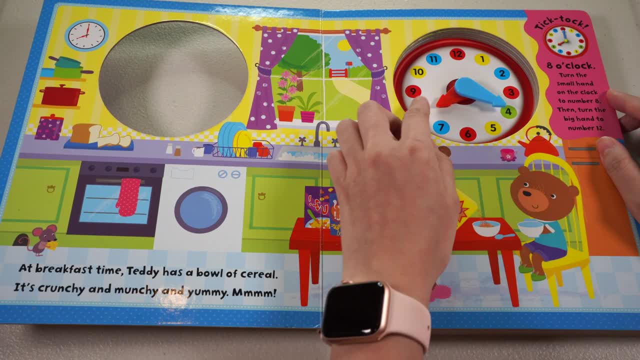 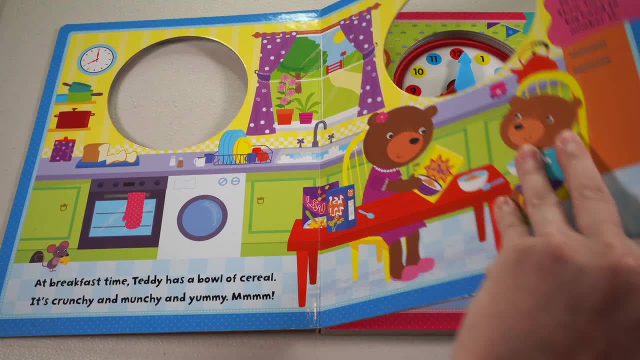 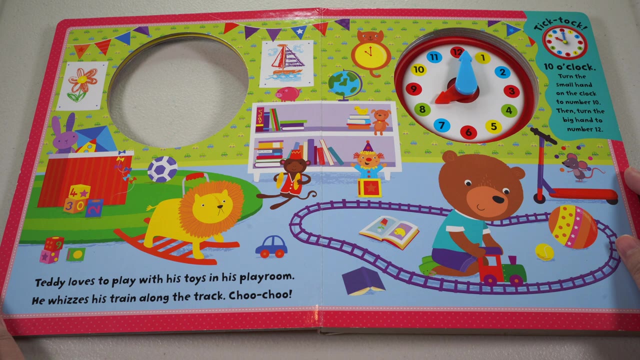 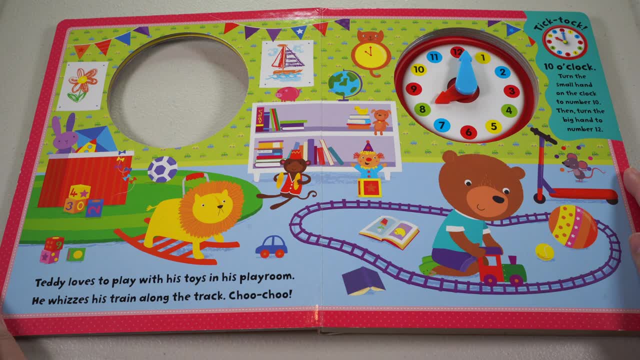 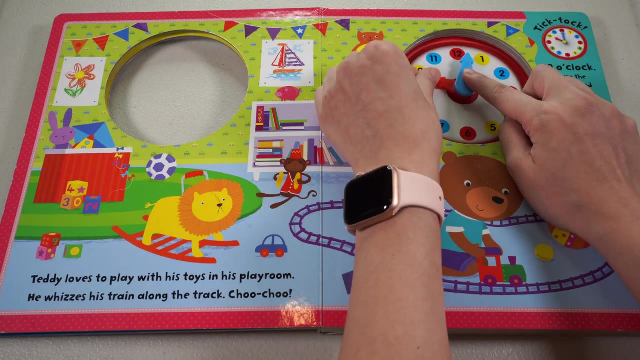 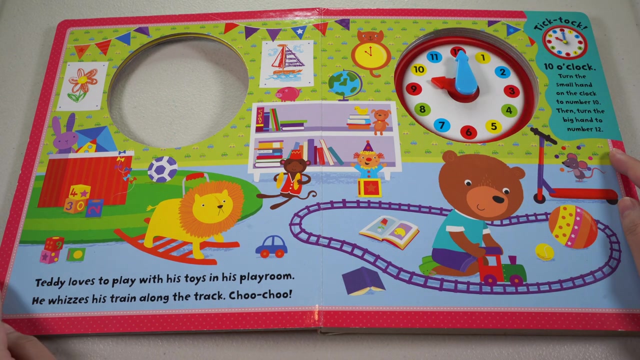 Choo, choo, Wee, weee, Wee, weee. Tick tock, tick, tock, tick, tock. It's ten o'clock. Turn the small hand on the clock to number ten. Then turn the big hand to number twelve. It's ten o'clock. 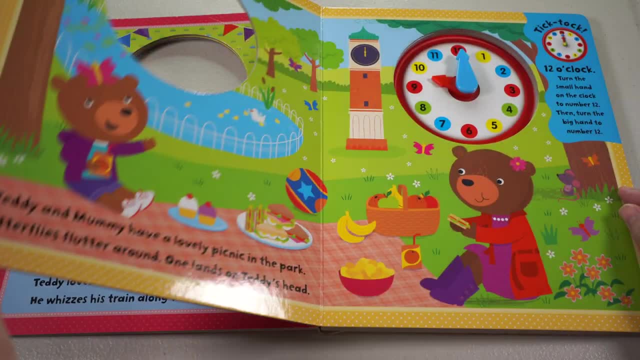 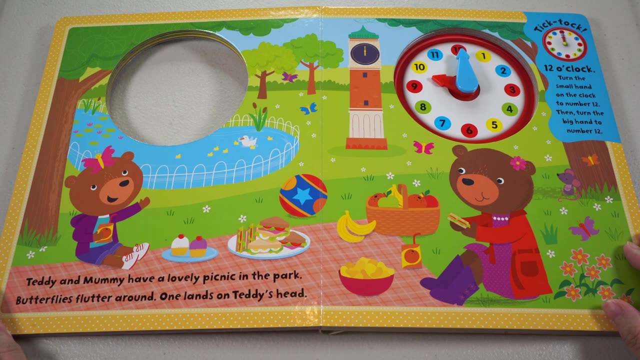 Teddy and Mommy have a lovely picnic in the park. Butterflies flutter around, One lands on Teddy's head. Tick tock, tick tock, tick tock. It's twelve o'clock. Turn the small hand on the clock to number twelve. Then turn the big hand to number twelve. 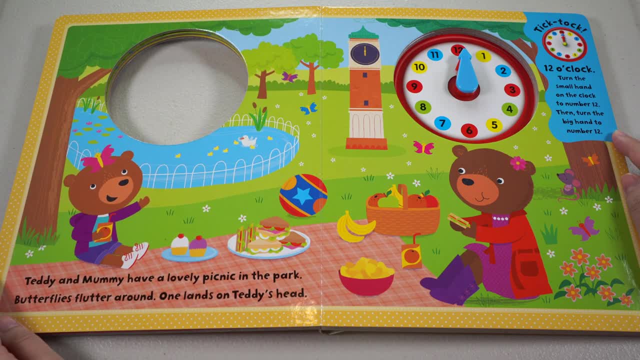 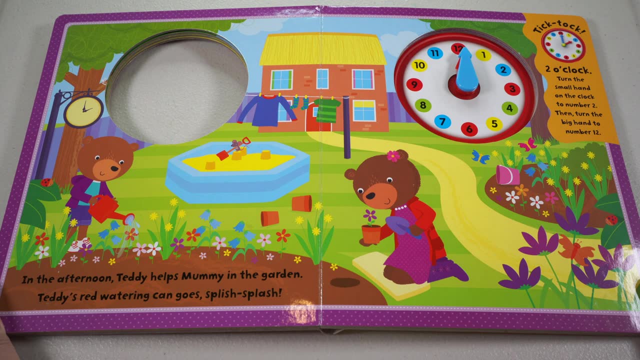 It's ten o'clock, Turn the big hand to number twelve. It's twelve o'clock. In the afternoon, Teddy helps Mommy in the garden. Teddy's red watering can goes splish, splash, Oh no. Tick tock, tick tock, tick tock. 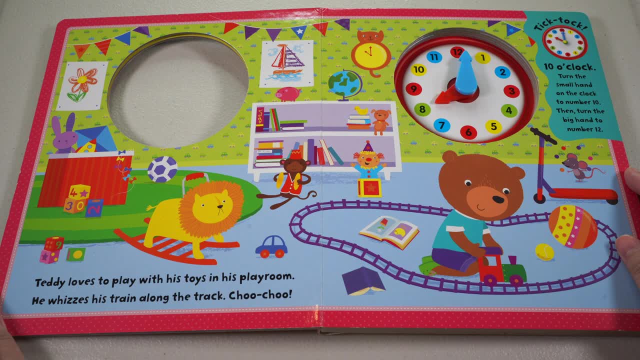 Teddy loves to play with his toys in his playroom. He whizzes his train along the track, Choo-choo, Tick-tock, tick-tock, tick-tock. It's ten o'clock. Turn the small hand on the clock to number ten. 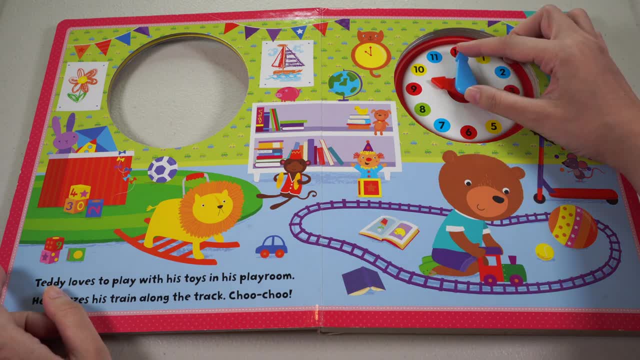 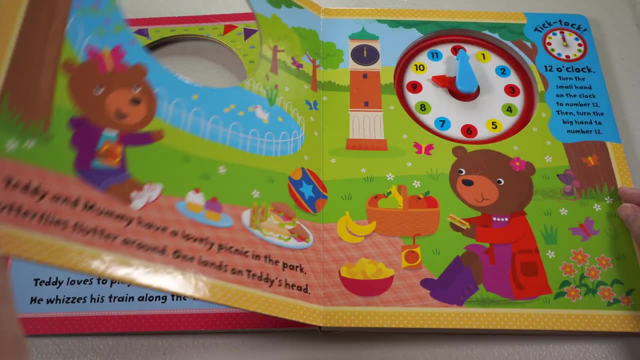 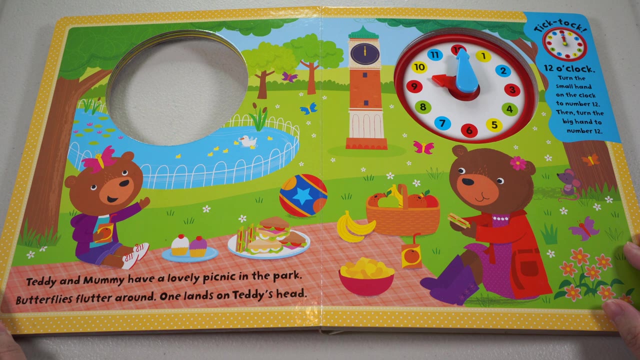 Then turn the big hand to number twelve. It's ten o'clock, Choo-choo. Teddy and Mommy have a lovely picnic in the park. Butterflies flutter around. One lands on Teddy's head, Tick-tock, tick-tock, tick-tock. 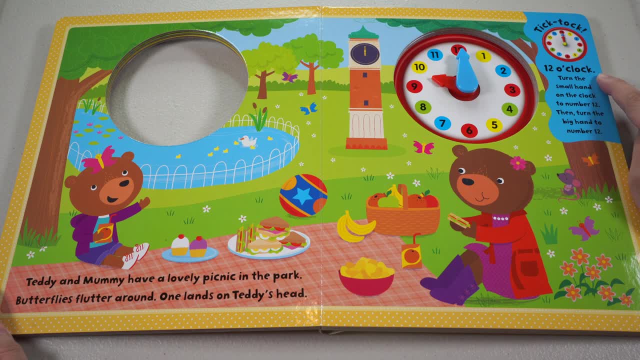 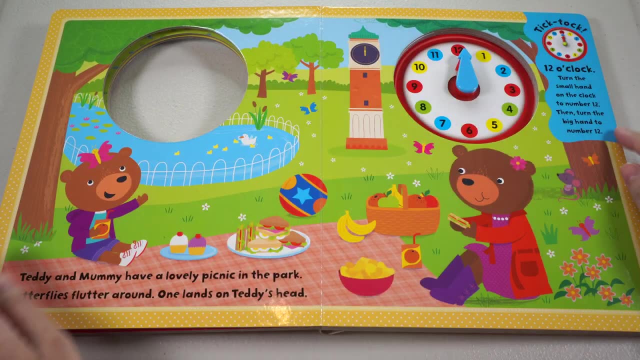 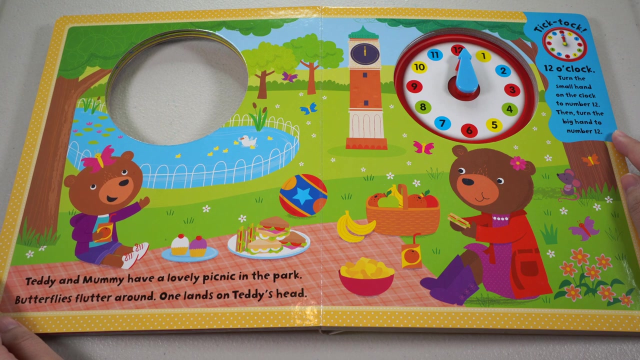 It's twelve o'clock. Turn the small hand on the clock to number twelve. Tick-tock, tick-tock, tick-tock. Then turn the big hand to number twelve. Turn the small hand on the clock to number twelve. It's twelve o'clock. 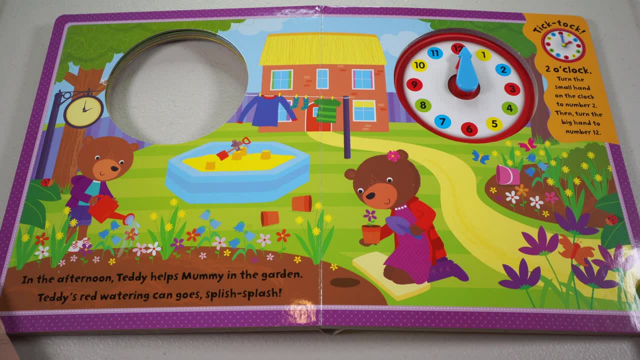 Choo-choo. In the afternoon, Teddy helps Mommy in the garden. Teddy's red watering can goes splish-splash. Oh no, Tick-tock, tick-tock, tick-tock. It's two o'clock. Turn the small hand on the clock to number twelve. 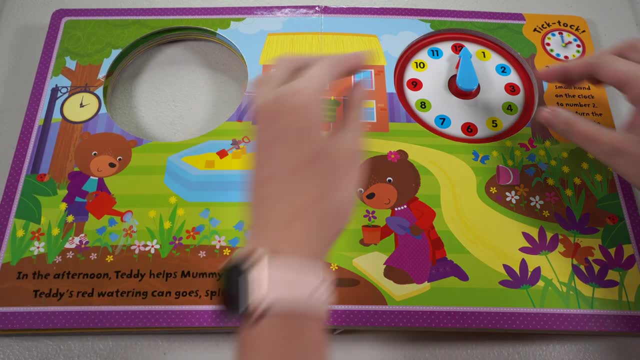 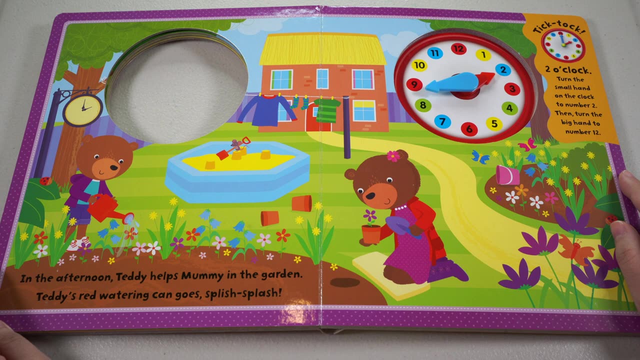 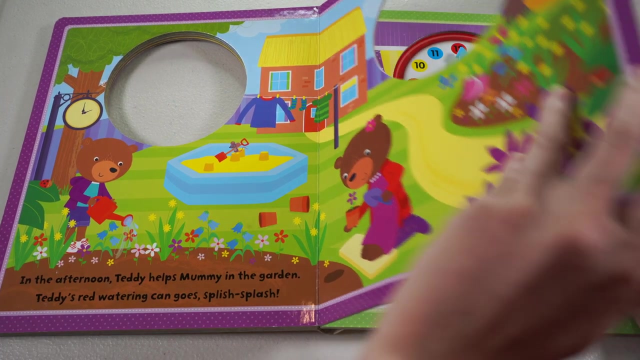 Turn the big hand on the clock to number two, Choo-choo. Then turn the big hand to number twelve, Choo-choo. It's two o'clock, Choo-choo, Choo-choo. 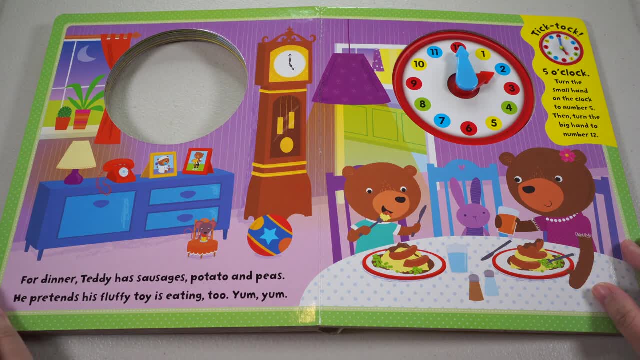 For dinner. Teddy has sausages, potatoes and peas. He pretends his fluffy toy is eating two eggs. Choo-choo eating too. Yum yum, Tick tock, tick, tock, tick tock, It's five o'clock. Turn the small. 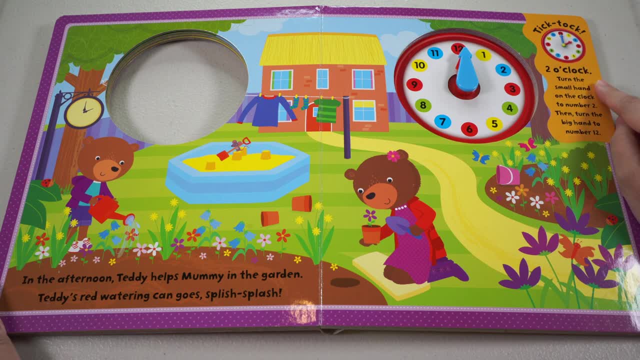 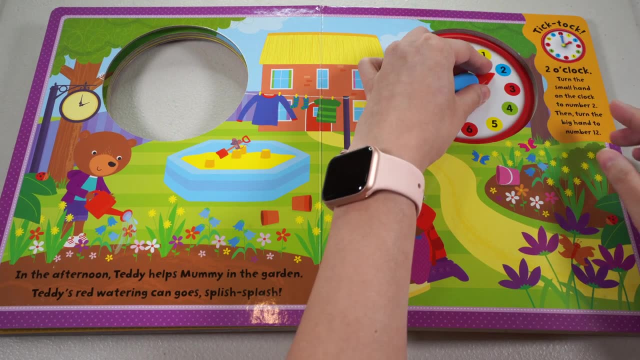 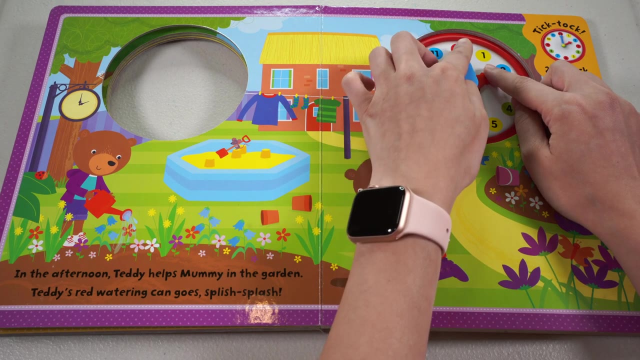 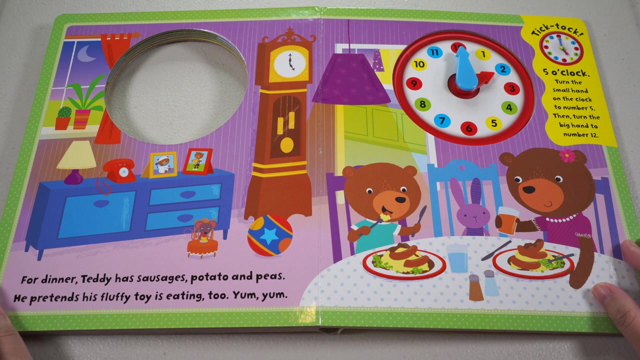 It's two o'clock, Turn the small hand on the clock to number twelve. Then turn the big hand on the clock to number two. Then turn the big hand to number twelve. It's two o'clock. For dinner, Teddy has sausages, potatoes and peas. 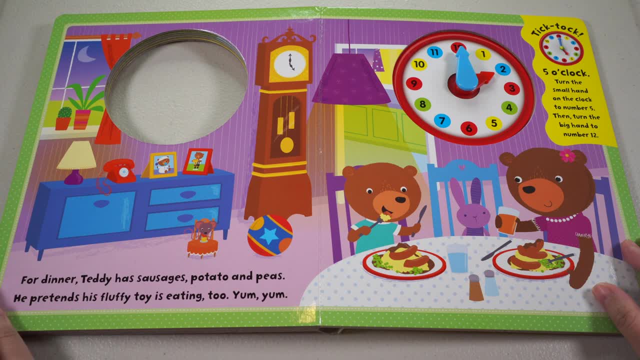 He pretends his fluffy toy is eating two pieces of cheese. He pretends his fluffy toy is eating two pieces of cheese, Yum yum, Tick tock, tick, tock, tick tock. It's five o'clock. Turn the small hand on the clock to number five. 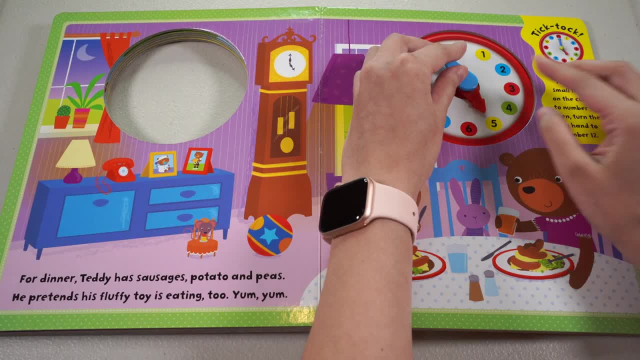 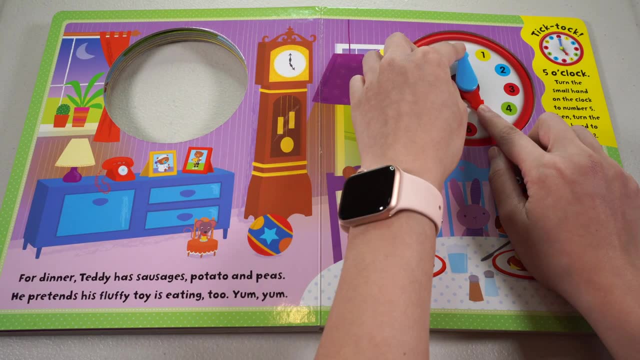 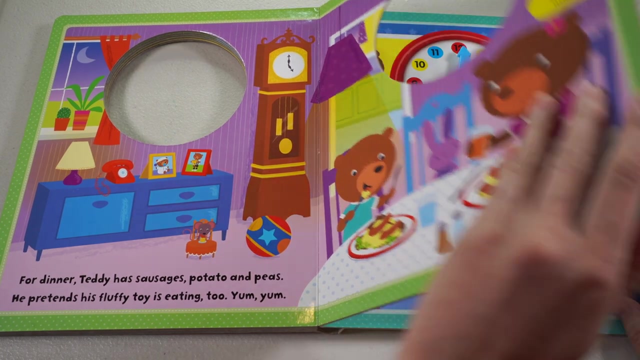 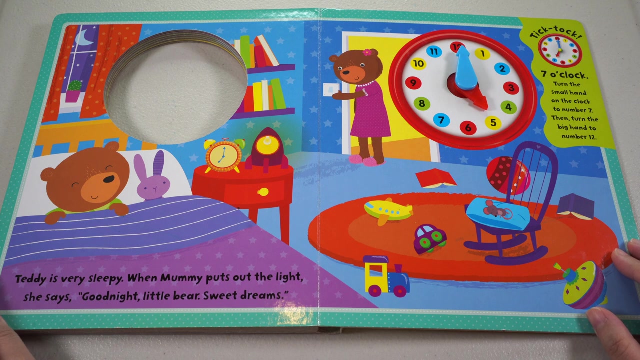 Then turn the big hand to number twelve. It's five o'clock. Teddy is very sleepy. when mommy puts out the light she says: good night, little bear, sweet dreams. tick tock, tick, tock, tick, tock. it's seven o'clock. turn the small hand on the clock to number seven. 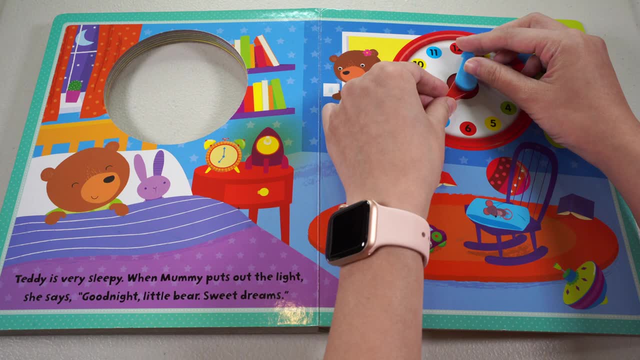 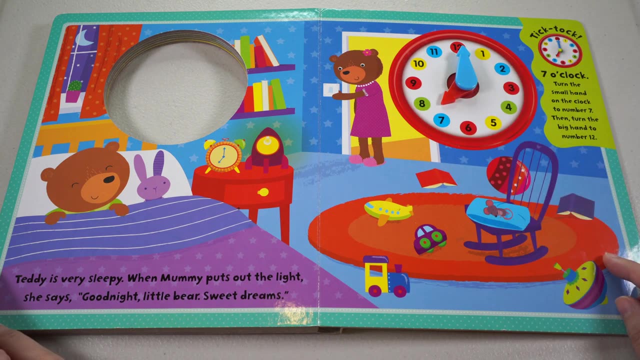 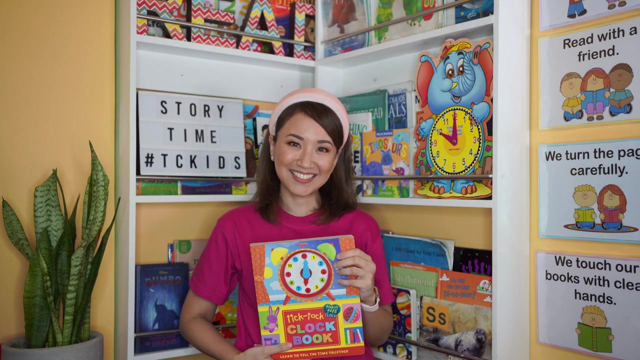 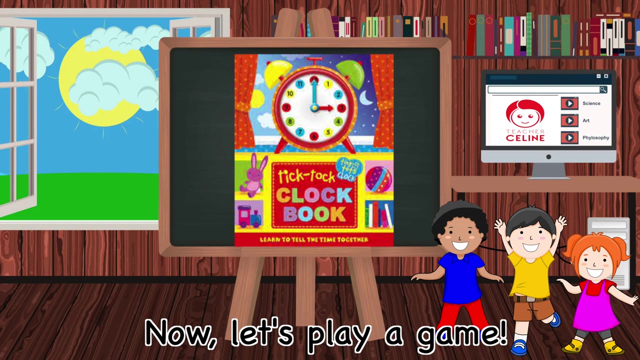 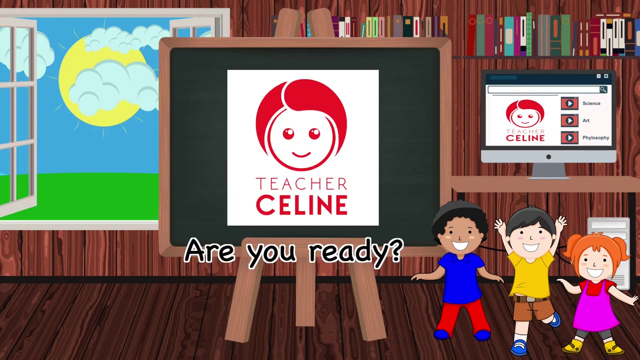 small hand there, then turn the big hand to number 12.. it's seven o'clock- the end. woohoo. did you guys enjoy our story for today? now let's play a game. tell me the time as soon as i flashed it on my screen. are you ready? okay, let's start. what time is it? 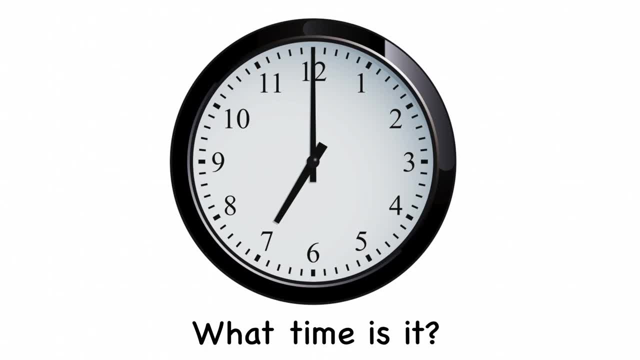 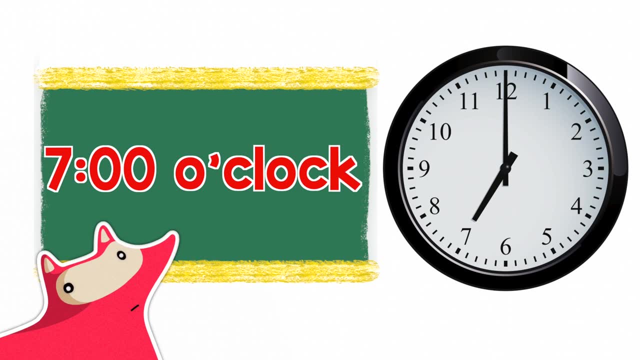 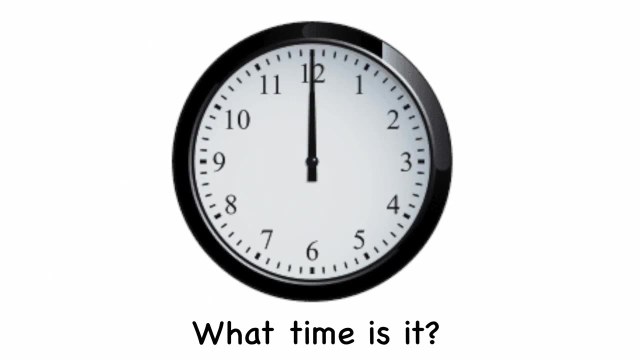 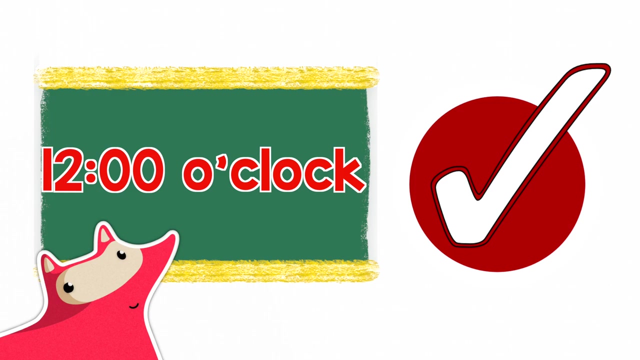 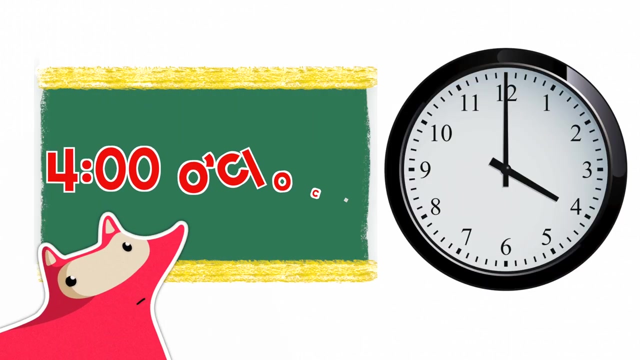 very good, it's 10 o'clock. what time is it? very good, it is seven o'clock, if you are correct. give yourself a check. next, what time is it that is correct again is 12 o'clock. how about this one? what time is it? yay, my tz kids are number smart. it's 4 o'clock next, how about this one? what time is it? yay that. 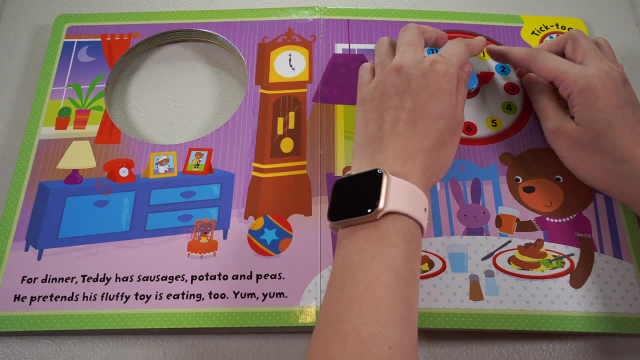 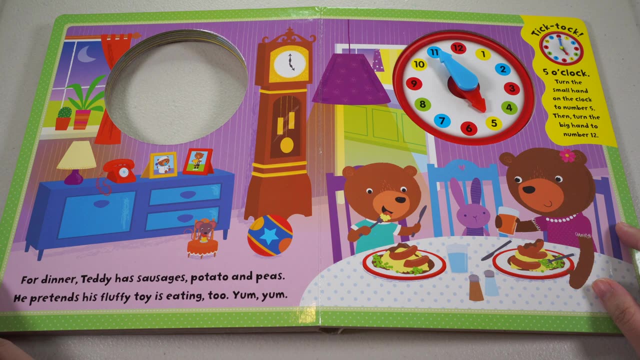 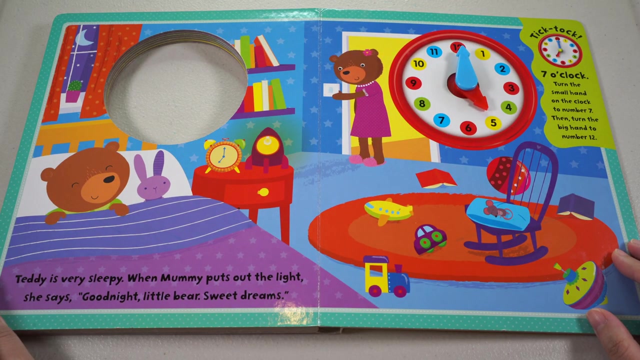 hand on the clock to number five. Small hand, There you go. Then turn the big hand to number twelve. It's five o'clock. Teddy is very sleepy. When mommy puts out the light she says: good night, little bear. Sweet dreams, Tick tock, tick tock. tick tock, It's seven. 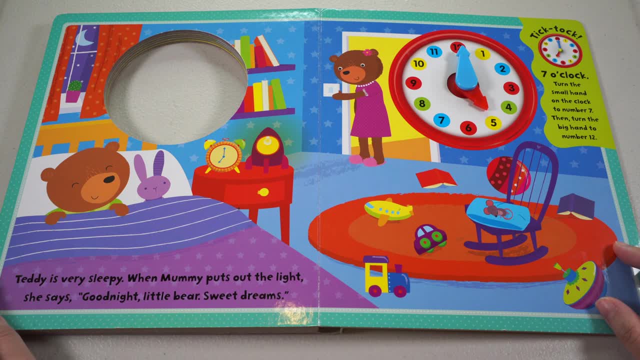 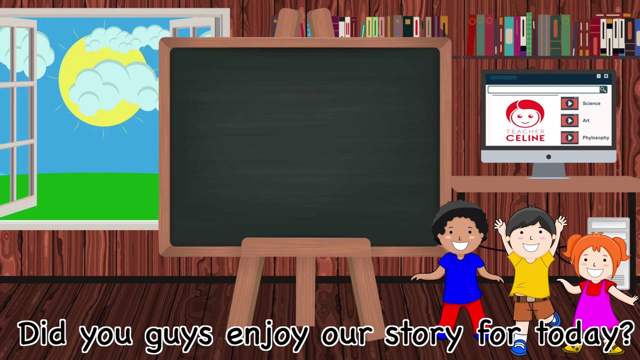 o'clock. Turn the small hand on the clock to number seven. Small hand there. Then turn the big hand to number twelve. It's seven o'clock The end. Woohoo, Did you guys enjoy our story for today? Yeah, Now let's play. 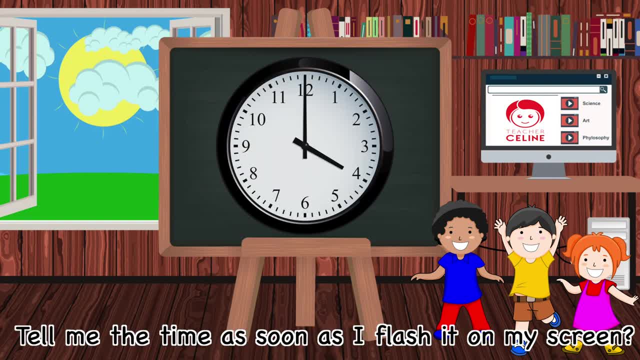 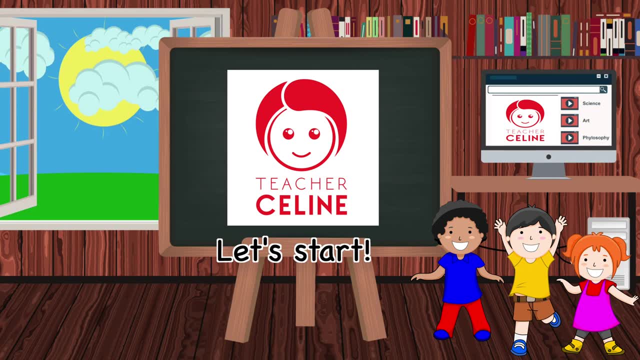 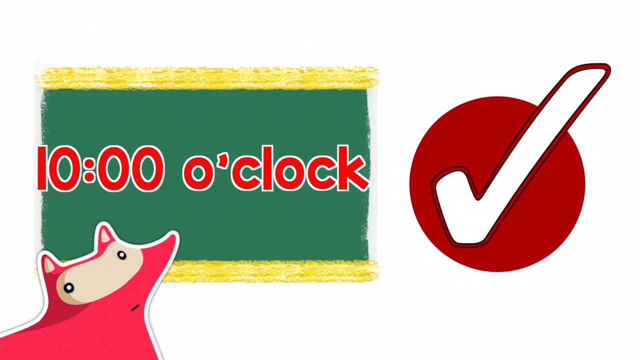 Let's play a game. Tell me the time as soon as I flashed it on my screen. Are you ready? Okay, let's start. What time is it Very good. It's ten o'clock, What time is it Very good. 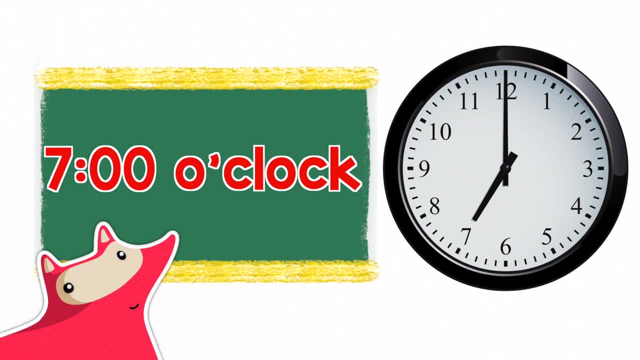 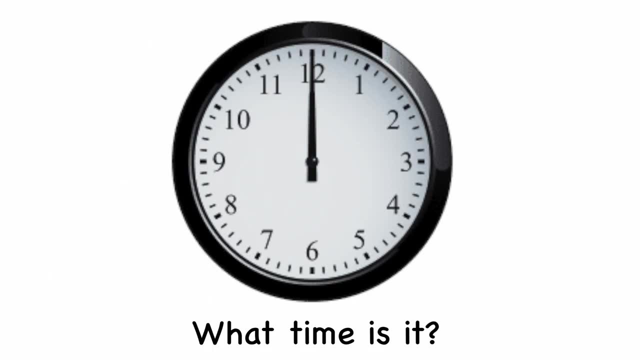 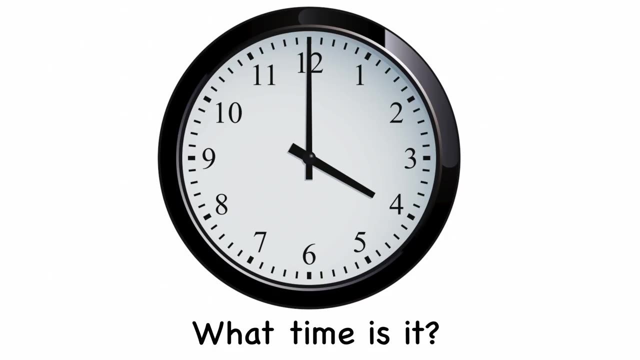 It is seven o'clock, If you are correct. give yourself a check. What time is it? The day of my birthday is today Eight o'clock. What about this TV? It seems to be left off today. This baby has nothing on the TV. Oh dear, it is just which day? 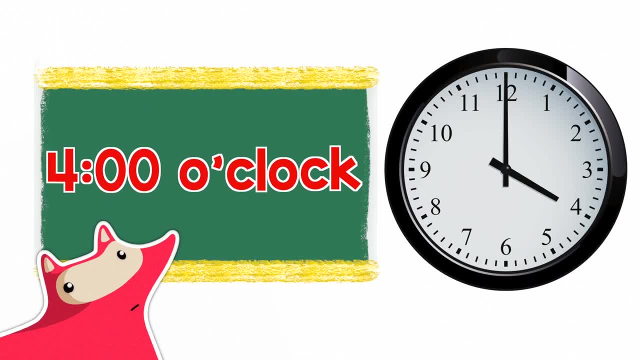 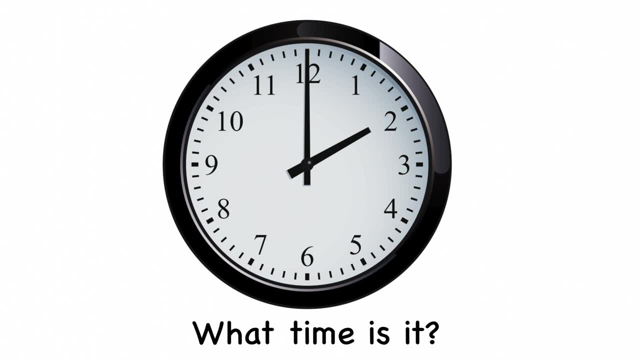 Hey, that's correct. The day it is now is six o'clock. Now, what time is it»? that is with the bene ph quanto calcio. what time is it? Is that correct? What's your answer? Next, what time is it? It's 12 o'clock". How about this one? What time is it? Yay, My TC Kids are number smart: It's four o'clock". What time is it? It's four o'clock. How about this one? What time is it? It's two o'clock. Sweet dreams, Kinder, or tiny noisesB shines' on their birthday Another май. sweet dreams, com'on. good night. 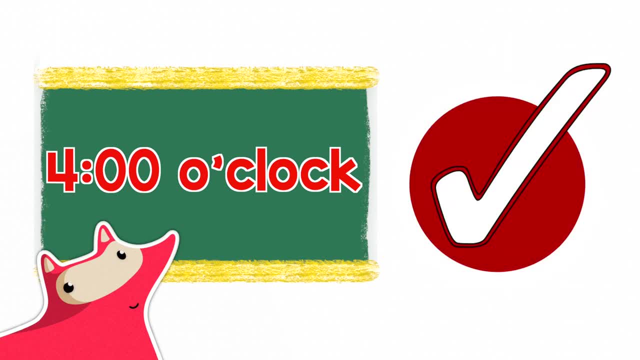 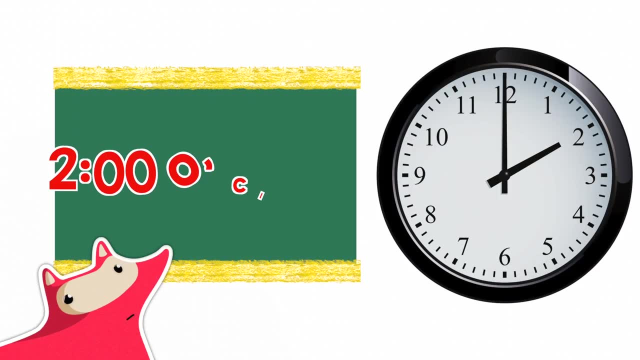 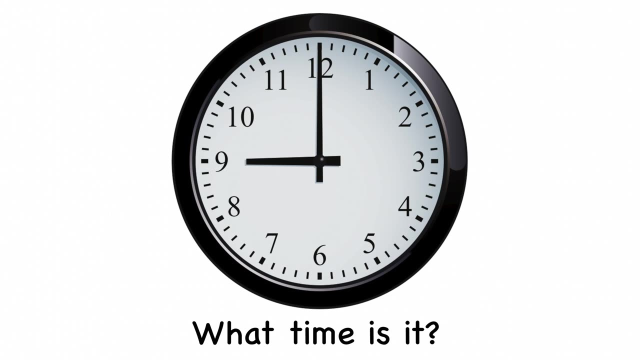 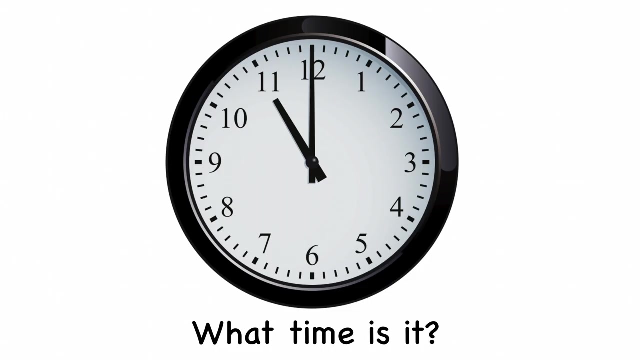 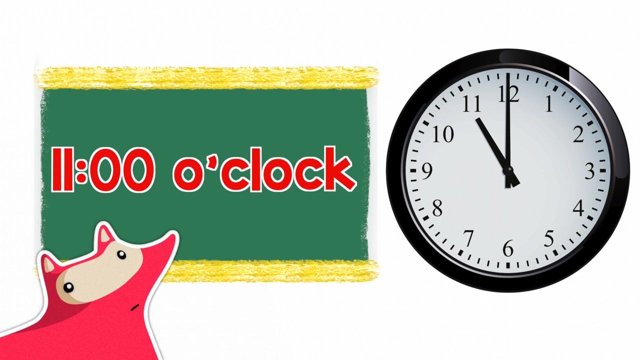 is correct, it's 2 o'clock. how about this one? what time is it? yay, that is correct. it's 2 o'clock. this one: what time is it that is correct? it's nine o'clock. last one: what time is it that is correct? again, it's 11 o'clock. if you are correct, give yourself a check. 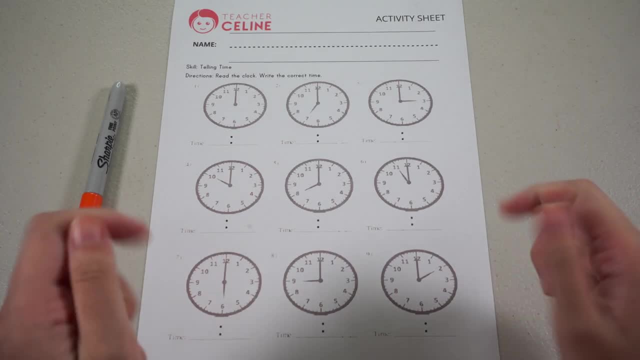 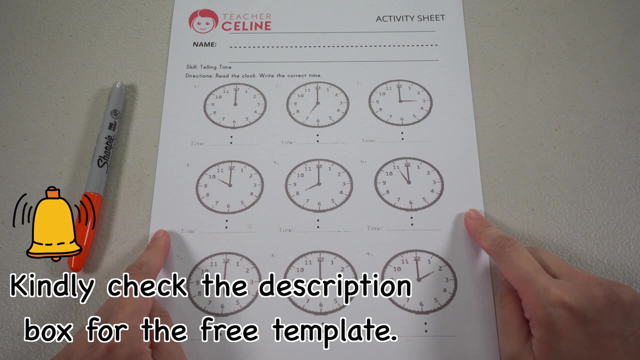 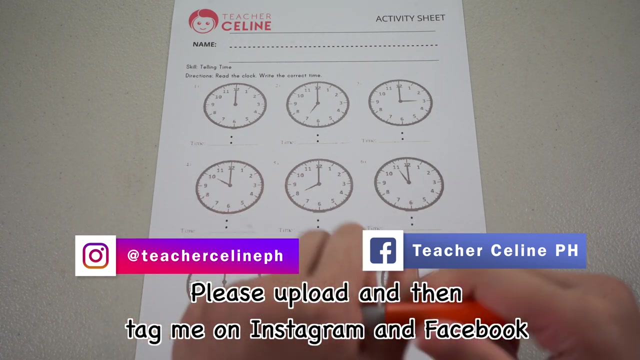 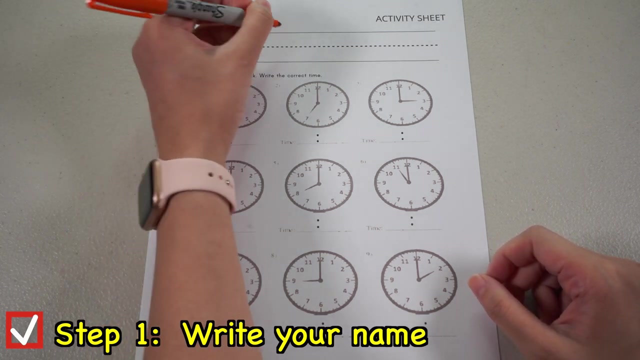 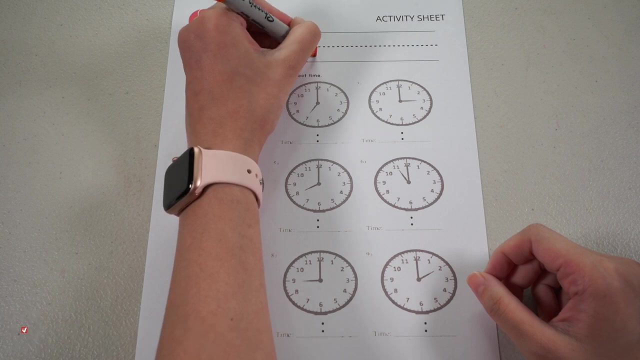 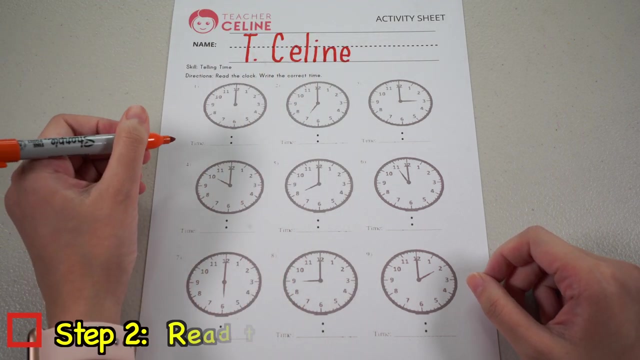 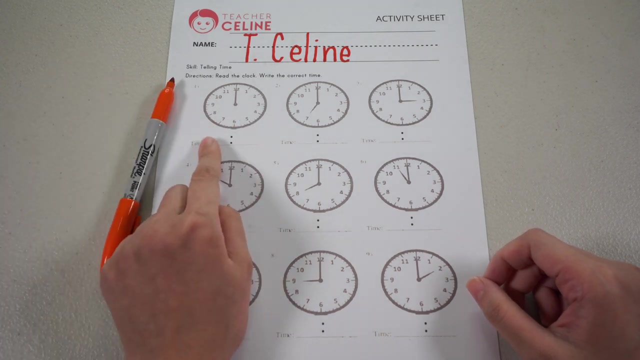 yay, we are now ready to answer our activity sheet. kindly check the description box to download the file. let's answer together: first is write your name. next let's read the directions. skill telling time directions. read the clock. write the correct time. let's look at number one: shorthand is pointing at 12 and longhand is pointing at 12 as well. 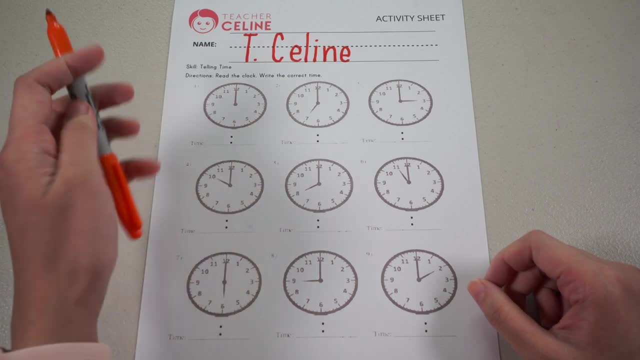 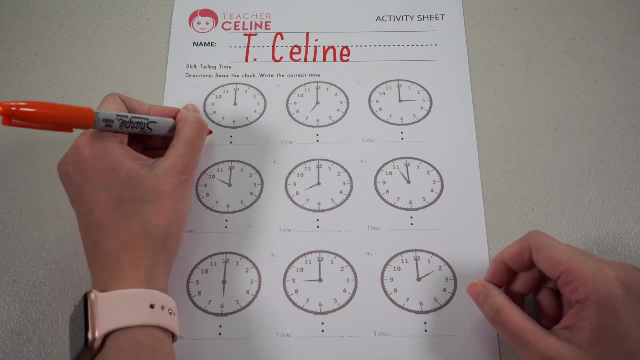 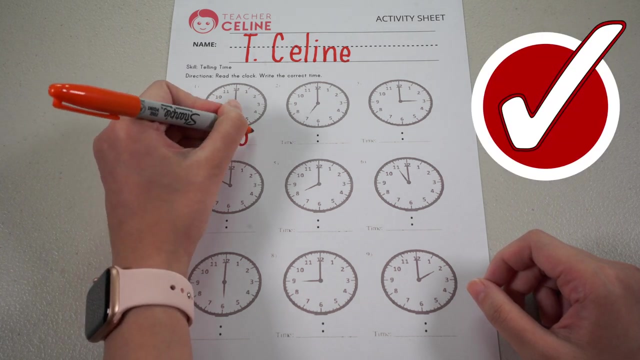 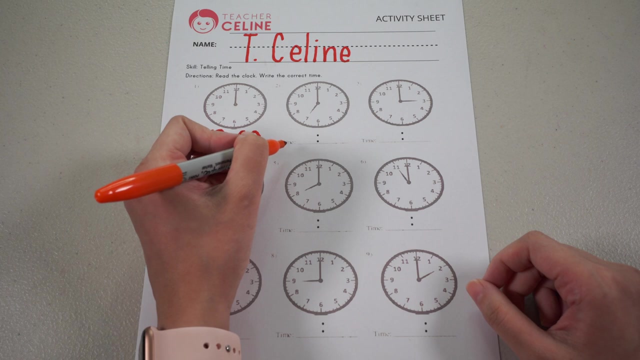 what time is it? very good, it's 12 o'clock. how do you write 12 o'clock? first, you write 12. when you see the longhand pointing at 12, you write zero, zero, 12 o'clock, very good. next: oh, what time is this? 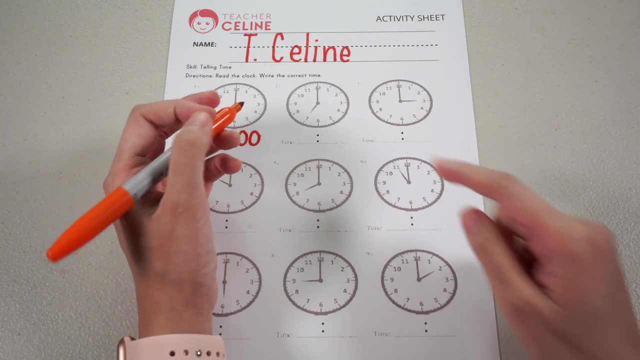 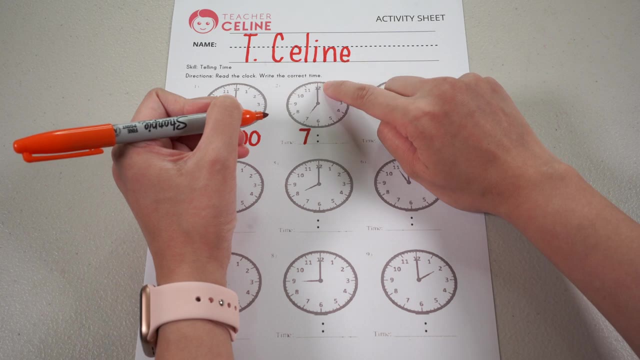 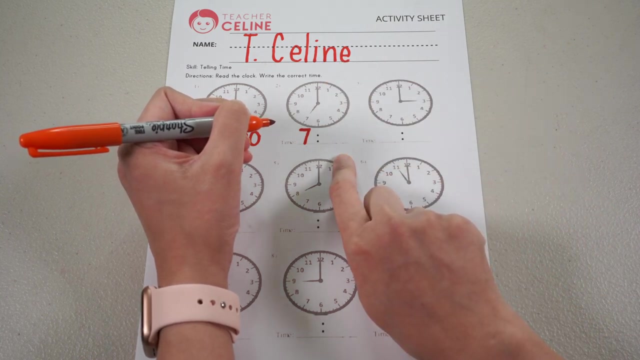 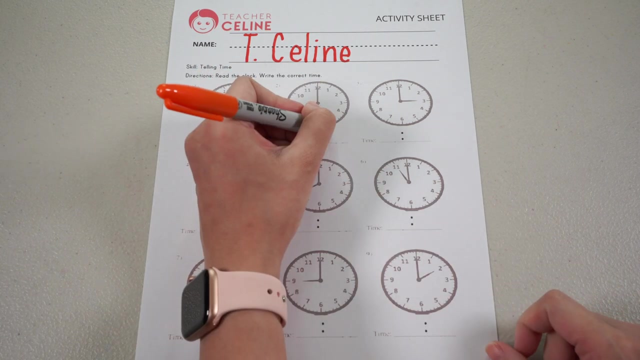 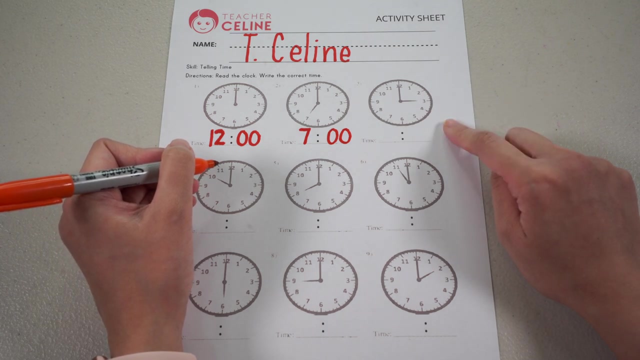 shorthand is pointing at seven, longhand is pointing at 12.. it's very good, seven o'clock. what numbers do you put here? huh, do you write number 12.. oh, you're right, five zero, zero, very good. next, what time is it? very good, that is correct, it's three o'clock. 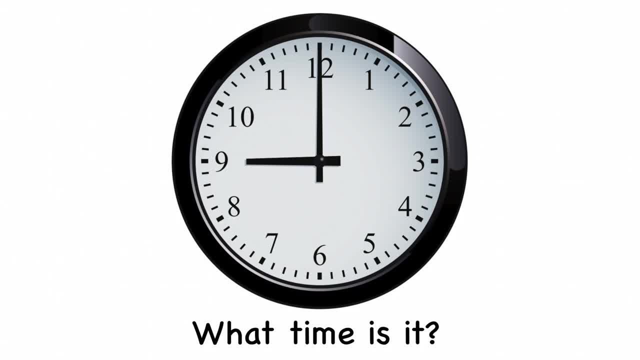 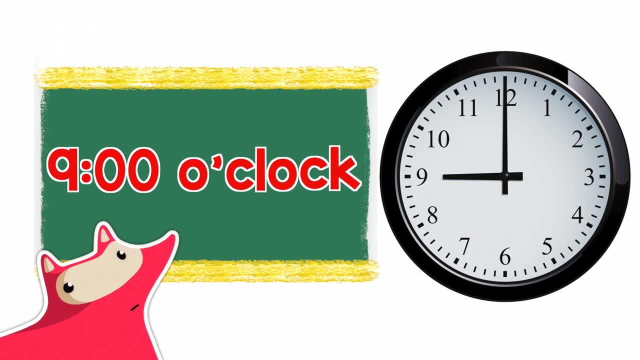 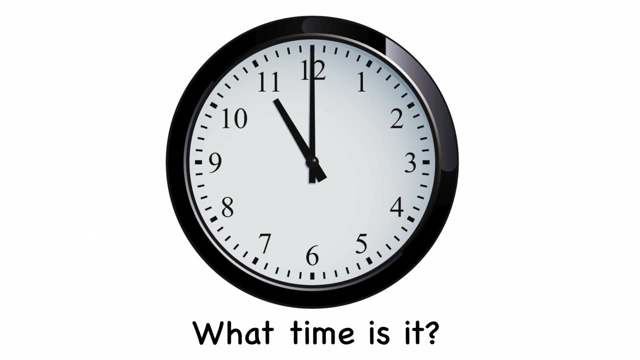 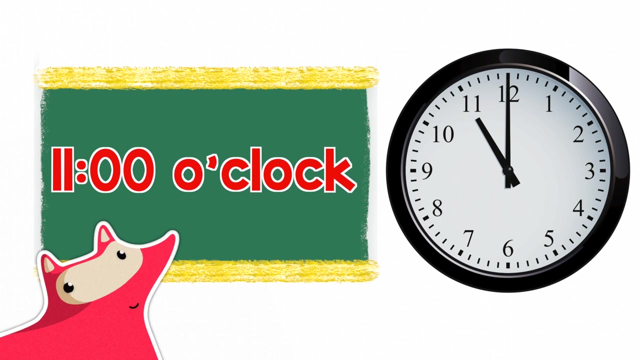 It's 2 o'clock. How about this one? What time is it That is correct? It's 9 o'clock. Last one: What time is it That is correct? again, It's 11 o'clock. If you are correct, give yourself a check. 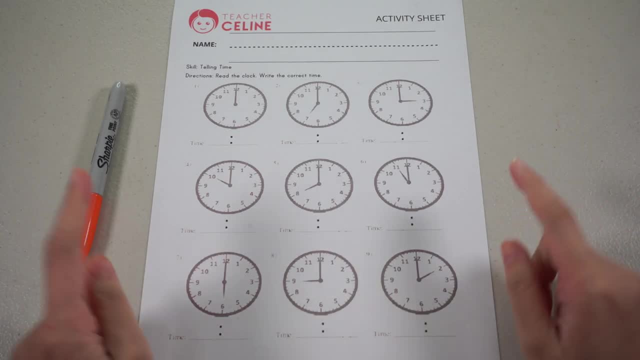 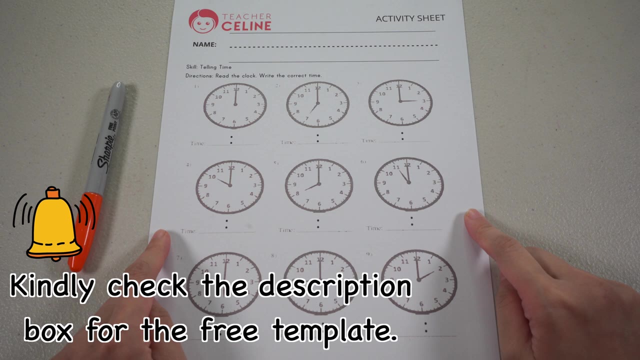 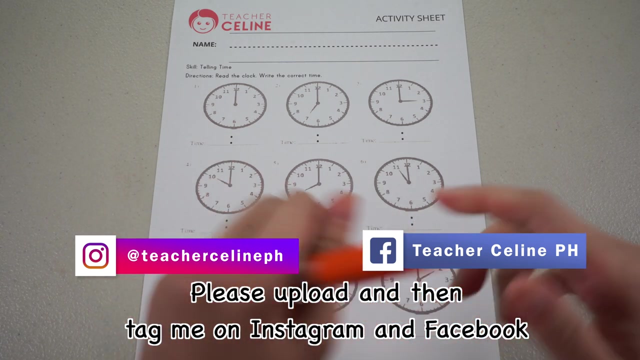 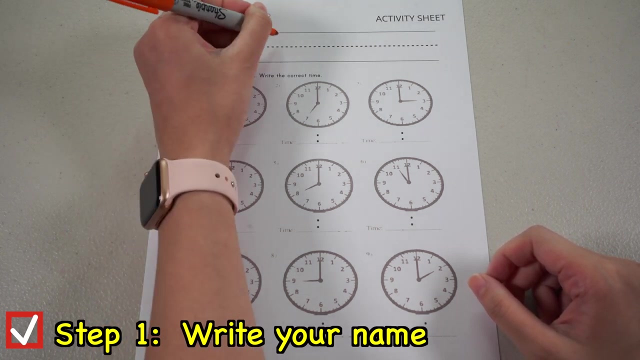 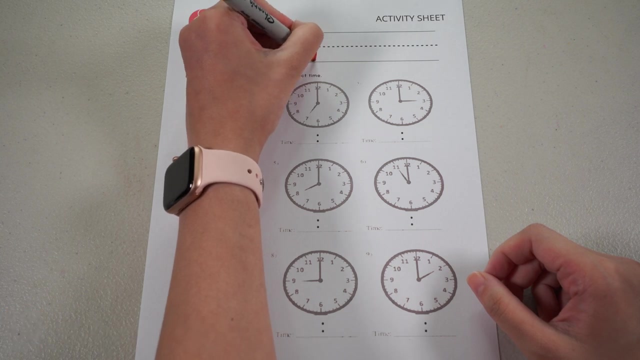 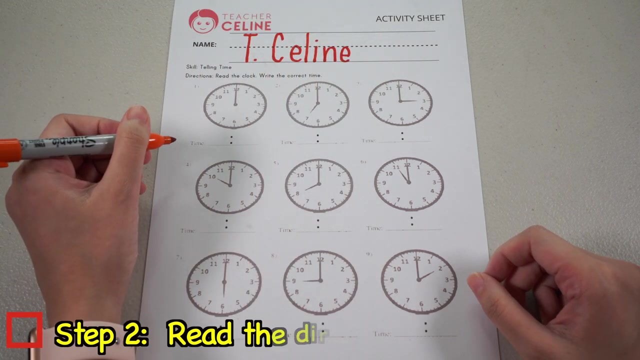 Cha-ching. Yay, We are now ready to answer our activity sheet. Kindly check the description box to download the file. Let's answer together. First is Write your name. Next let's read the directions. Skill Telling time Directions. Read the clock. Write the correct time. 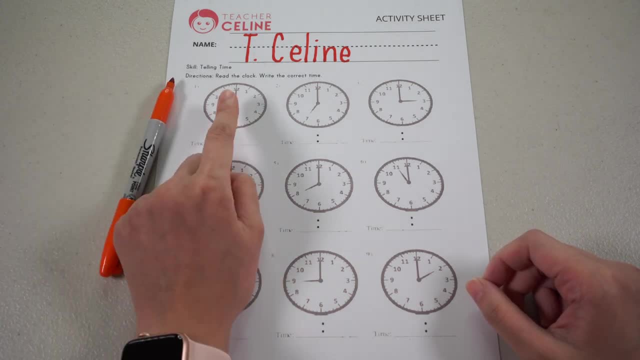 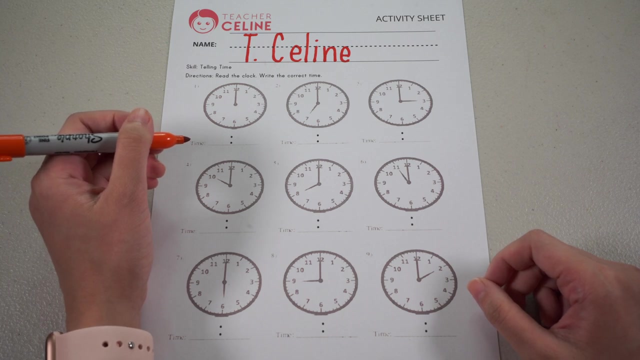 Let's look at number 1. Short hand is pointing at 12, Long hand is pointing at 12 as well. What time is it? Very good, It's 12 o'clock. How do you write 12 o'clock First you write 12. 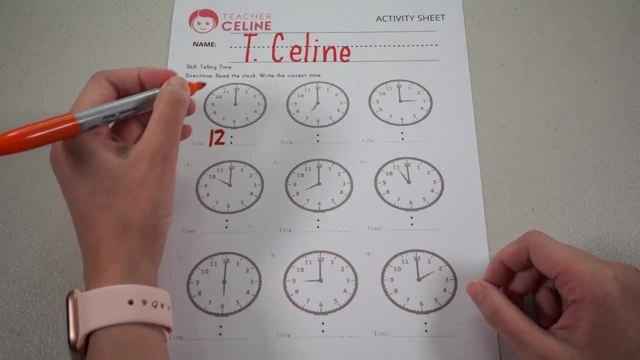 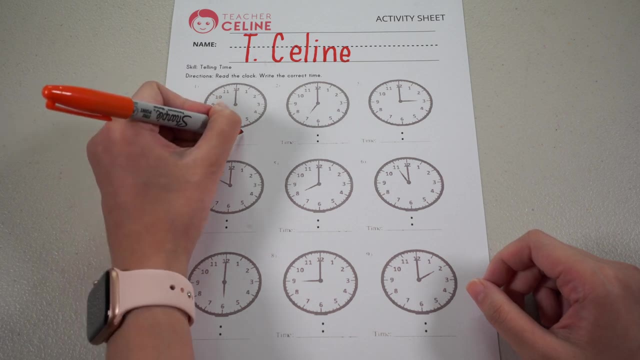 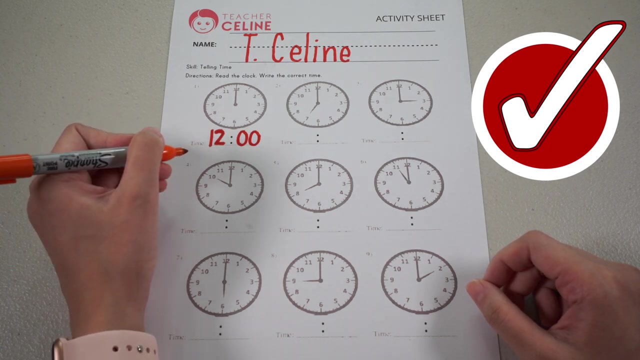 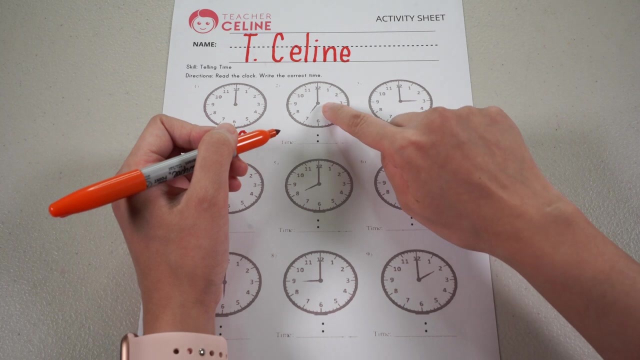 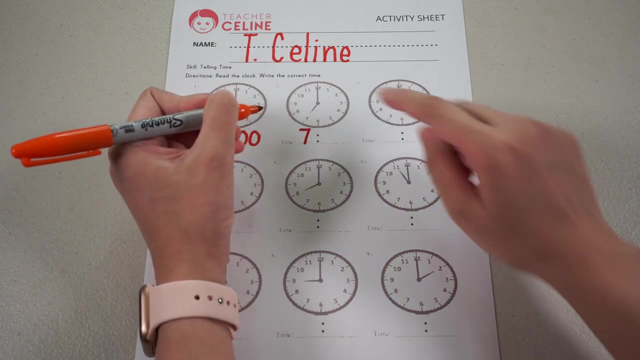 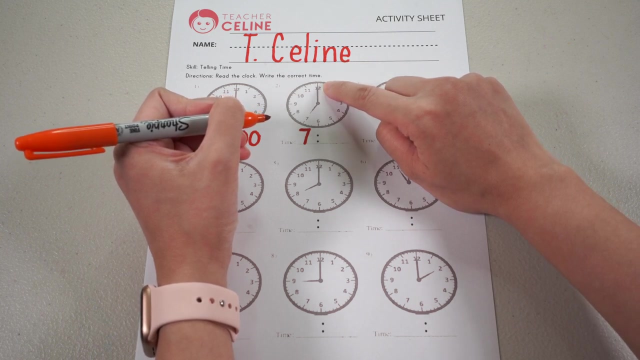 When you see the long hand pointing at 12, You write 00, 12 o'clock, Very good. Next, Oh, What time is it? What time is this? Short hand is pointing at 7. Long hand is pointing at 12. It's very good. 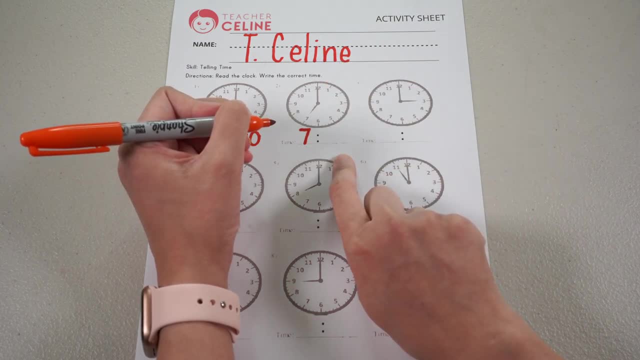 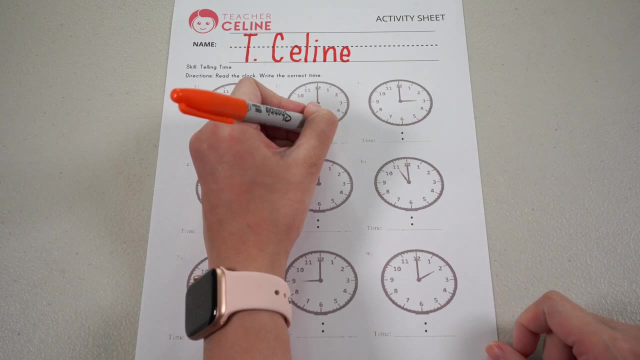 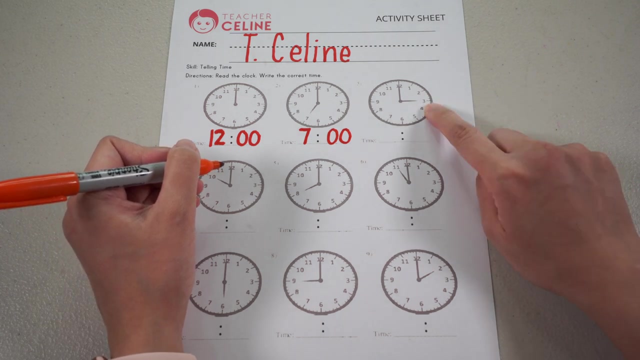 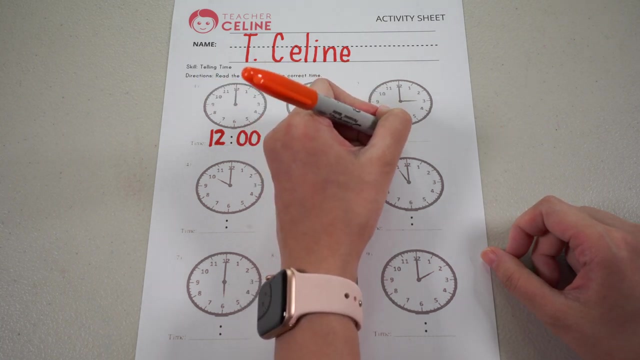 7 o'clock. What numbers do you put here? Do you write number 12?? Oh, you write 0, 0, Very good. Next, What time is it? Very good, That is correct, It's 3 o'clock, So write 3 Dot dot. 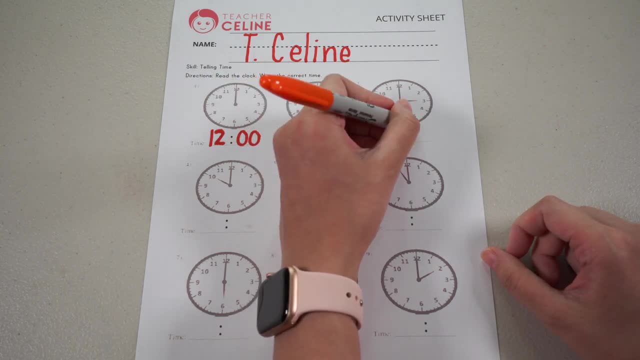 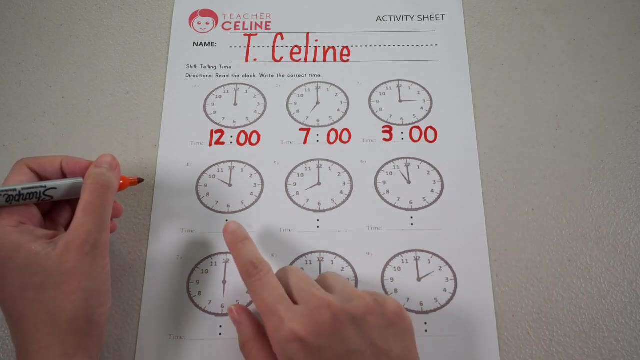 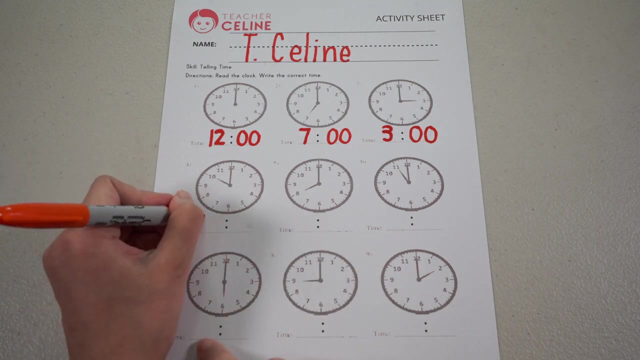 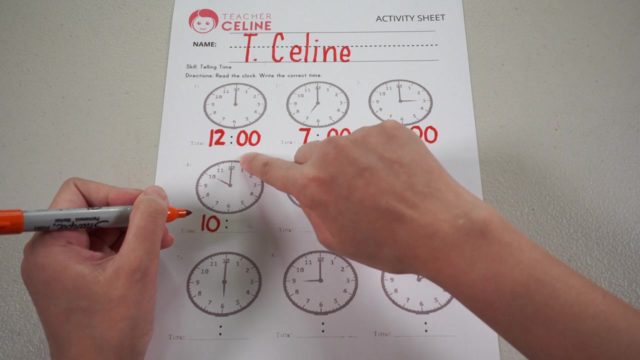 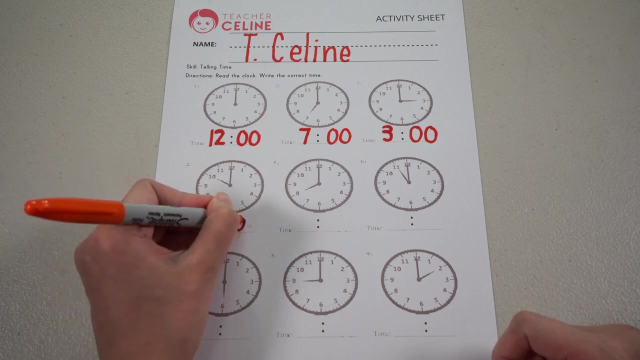 so write: three dot dot zero, zero. three o'clock next. what time is it? shorthand is pointing at 12.. 10 and longhand is pointing at 12.. it's 10 o'clock, so it's 10 dot dot, zero, zero. very good next. 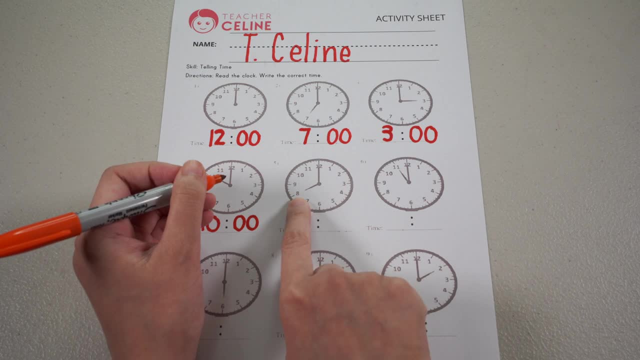 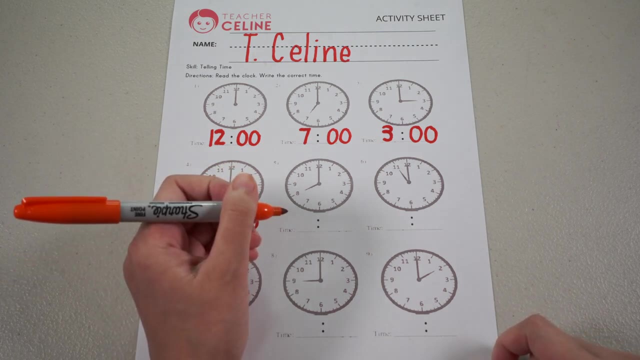 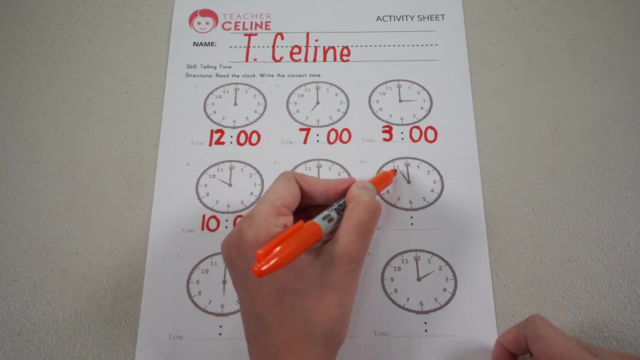 oh, what time is it? it's what number is this? very good, it's eight o'clock. how do you write eight o'clock? first write the number eight dot dot. then it's very good: zero and zero. next shorthand is pointing to what number? very good, it's eleven dot dot. 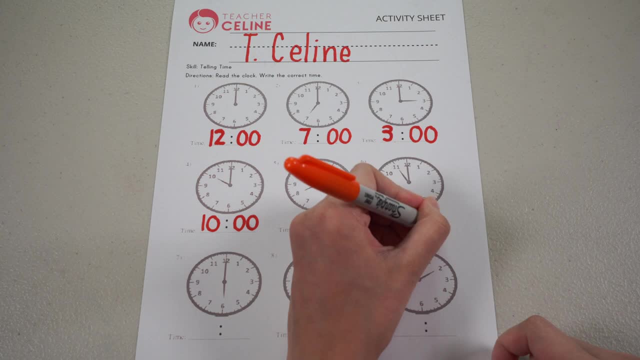 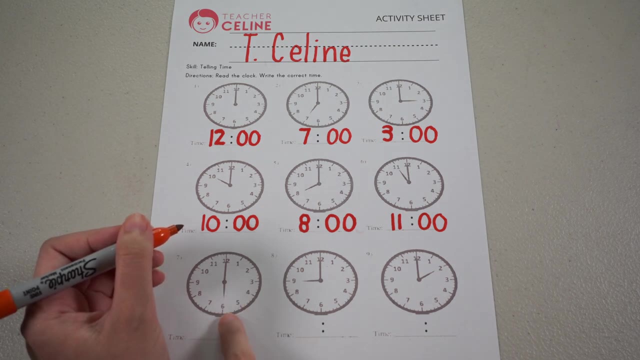 good, zero. zero, eleven o'clock next. what time is it? look at the shorthand. it's pointing at number. great job, six dot dot, that's correct. zero. what's next? another zero, six o'clock next. what time is it? yay, that is correct. you write nine dot dot. how many zeros? yes, two. 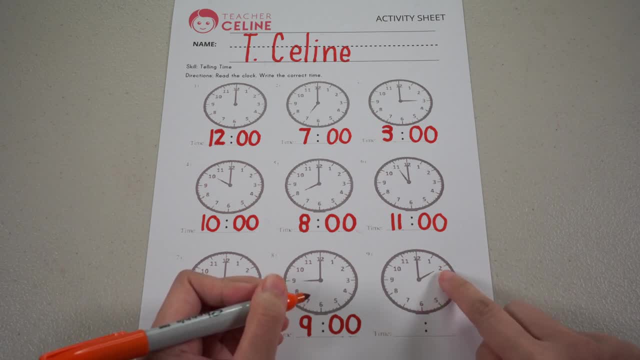 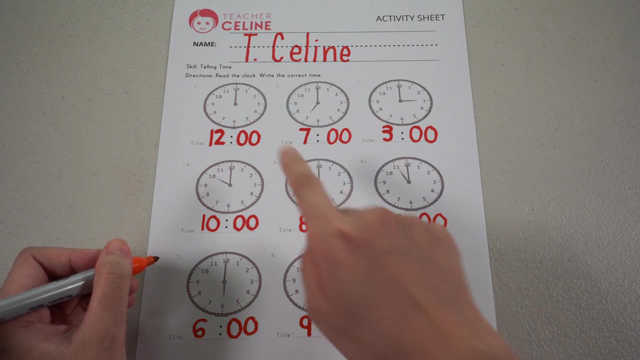 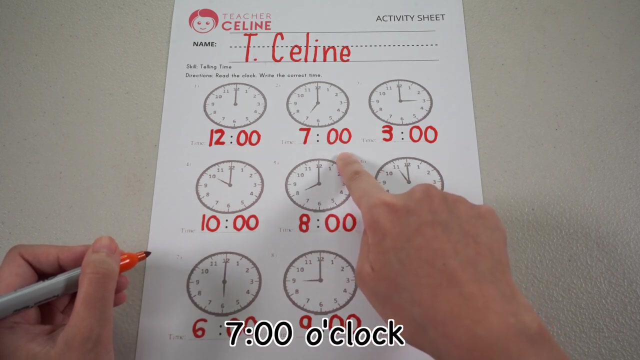 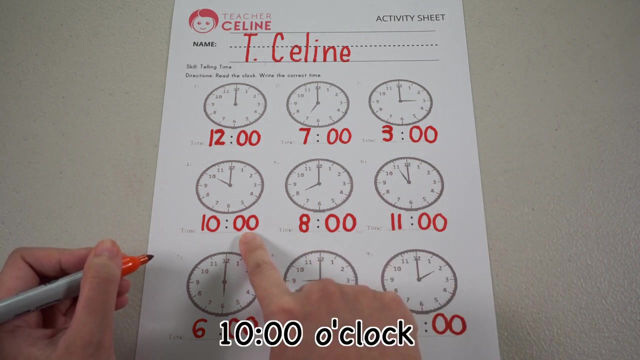 zeros. last one, what time is it? what number is this? very good, it's number two. dot dot, zero, zero. let's read one more time. what time is this? 12 o'clock next. seven o'clock, three o'clock, this one. ten o'clock, eight o'clock. how about this one? eleven o'clock next. 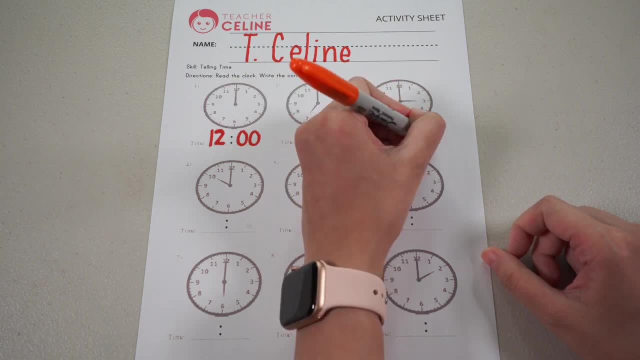 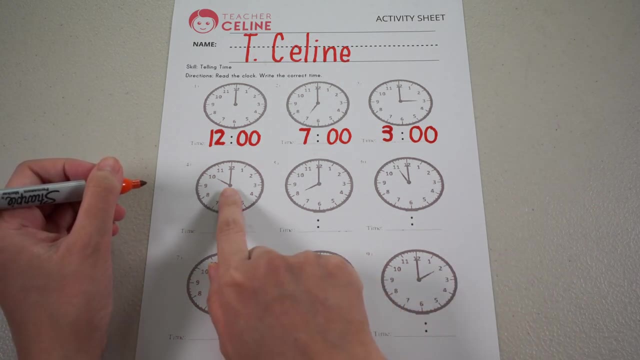 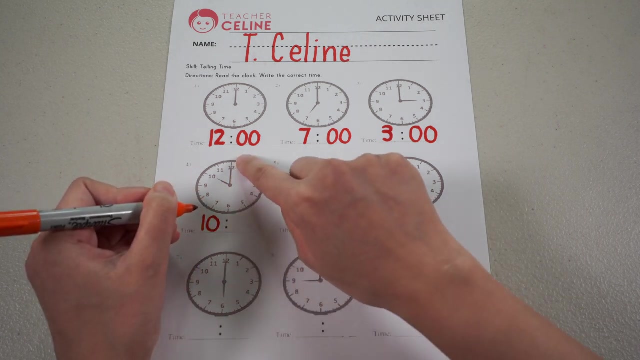 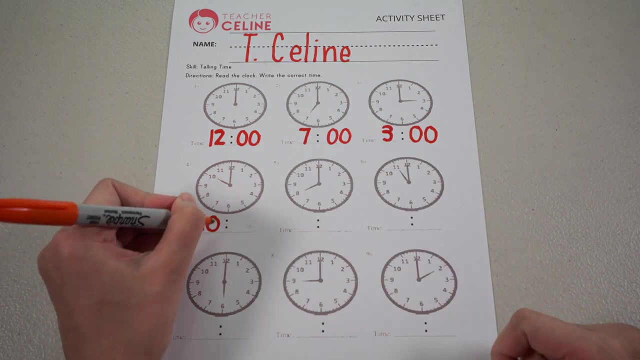 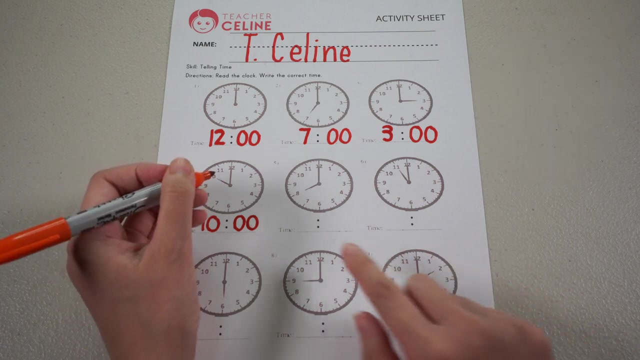 0, 0, 3 o'clock. Next. What time is it? Short hand is pointing at 10 And long hand is pointing at 10. long hand is pointing at 12. it's 10 o'clock, so it's 10, dot, dot, zero, zero, very good. next. 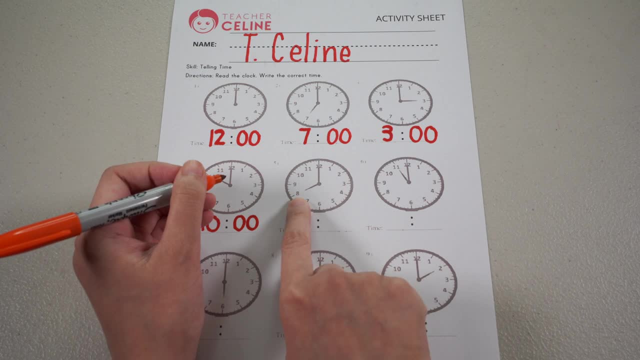 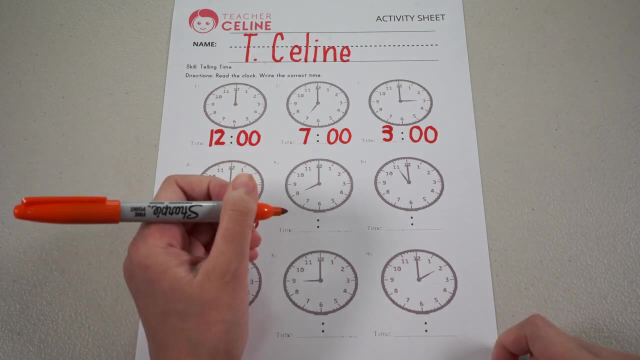 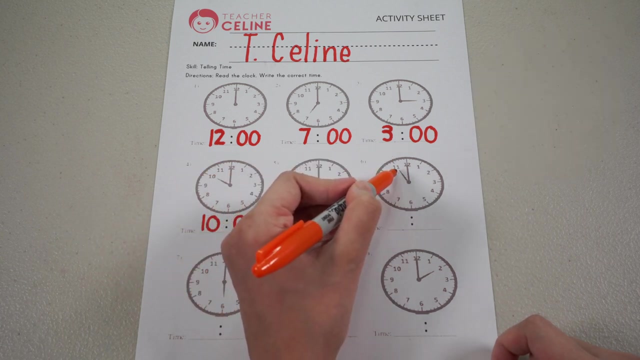 oh, what time is it? it's what number is this? very good, it's eight o'clock. how do you write eight o'clock? first write the number eight dot dot. then it's very good: zero and zero. next shorthand is pointing to what number? very good, it's eleven dot dot. 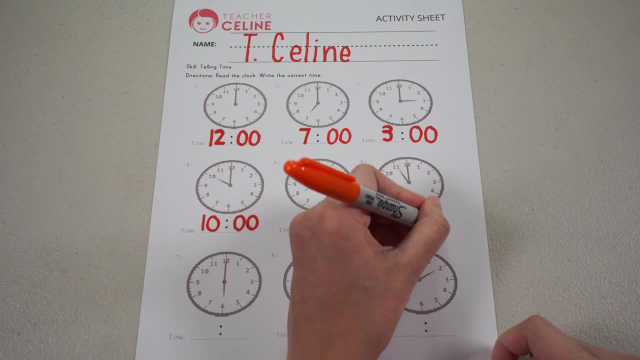 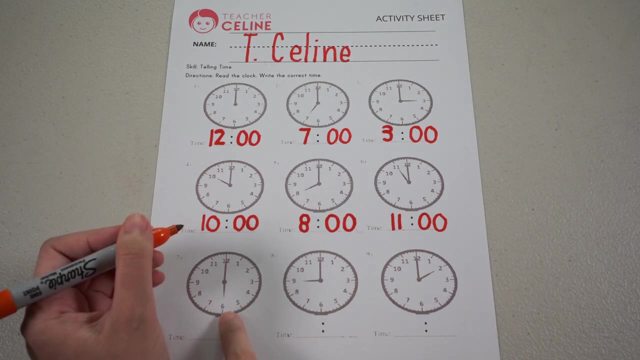 good, zero. zero, eleven o'clock next. what time is it? look at the shorthand. it's pointing at number. great job, six dot dot, that's correct. zero. what's next? another zero, six o'clock next. what time is it? yay, that is correct. you write nine dot dot. how many zeros? yes, two. 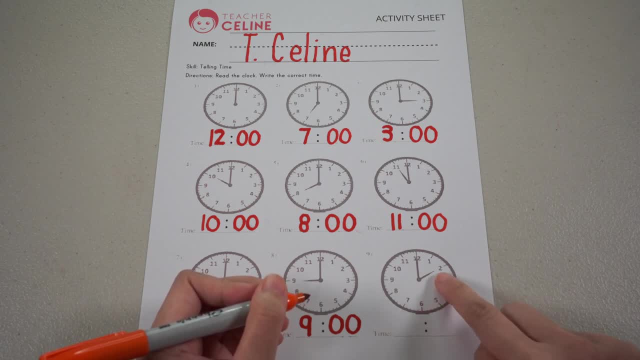 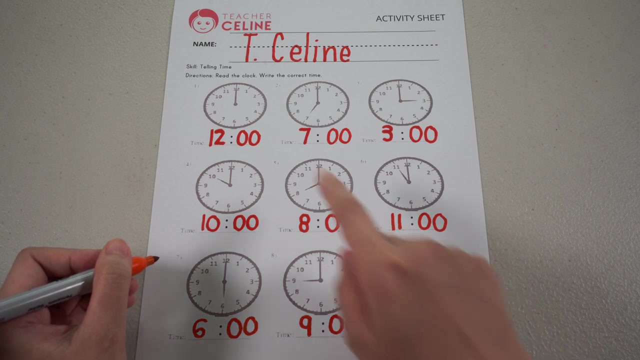 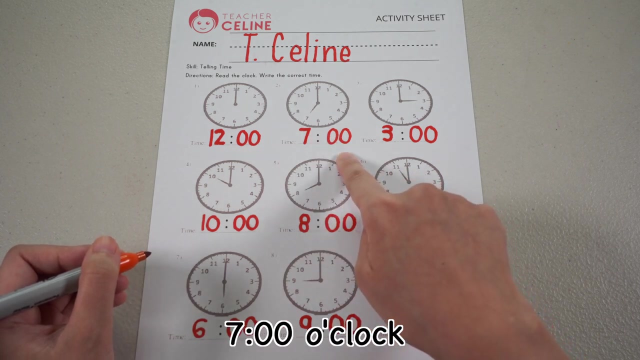 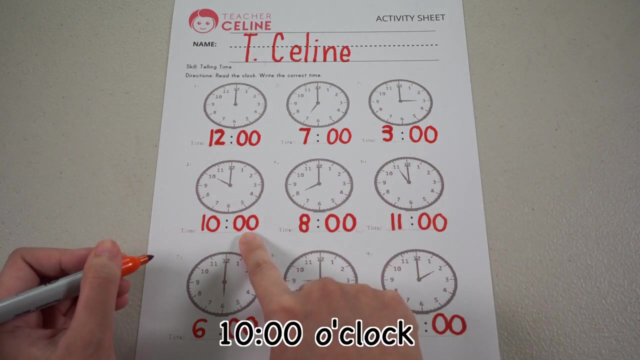 zeros. last one, what time is it? what number is this? very good, it's number two. dot dot, zero, zero. let's read one more time. what time is this? twelve o'clock, next, seven o'clock, three o'clock, this one. ten o'clock, eight o'clock about this one, eleven o'clock, next six o'clock.